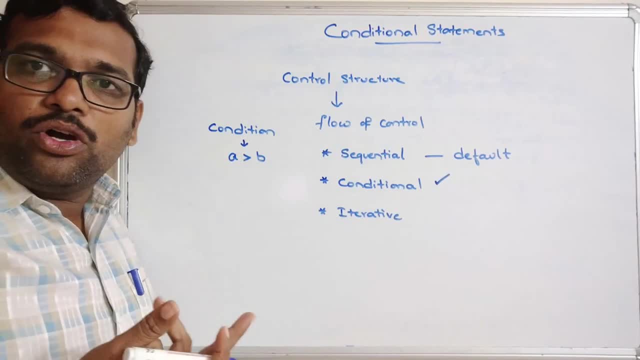 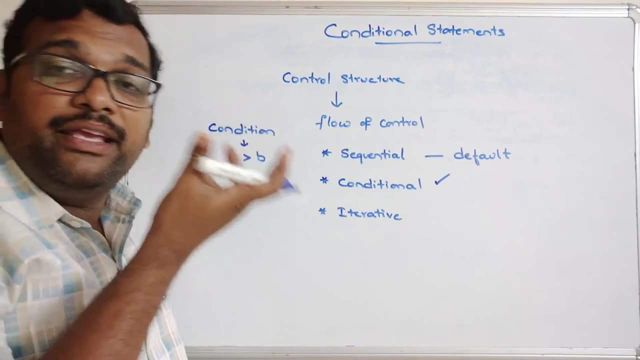 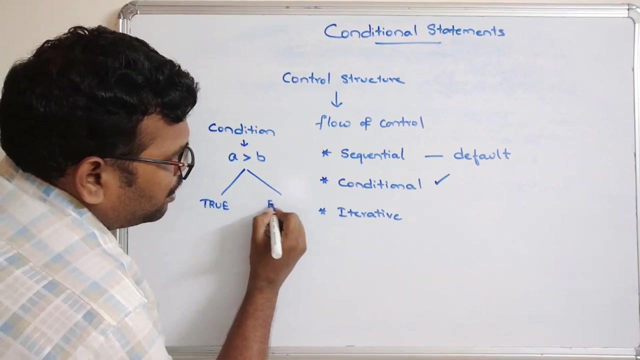 a greater than b is nothing but an condition, because a and b are operate operands and this is a relational operator. so we are comparing the values of a and b and the result will be either true or false, so which we call it as a boolean result. which we call it as a boolean result. so 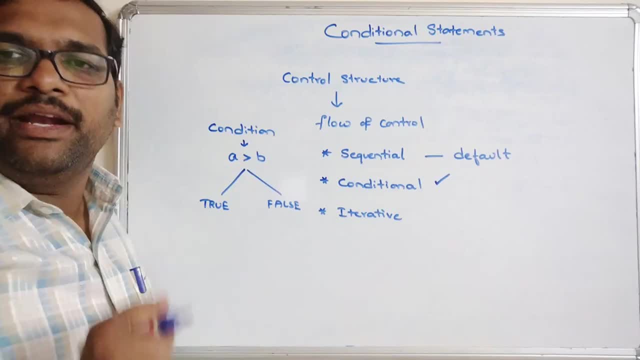 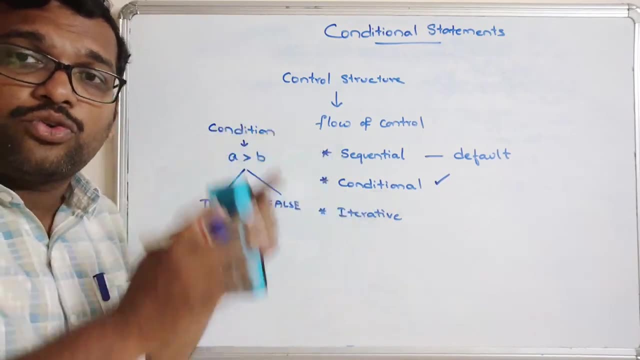 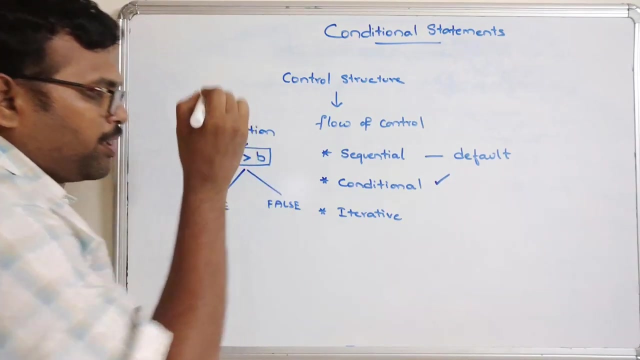 always the condition will result, a boolean result. that means either it will be true or false. so if you compare in the two variables, that result will be either true or it may be false, but not both right. so, based upon the result of this condition, based upon the result of this condition, the interpreter. 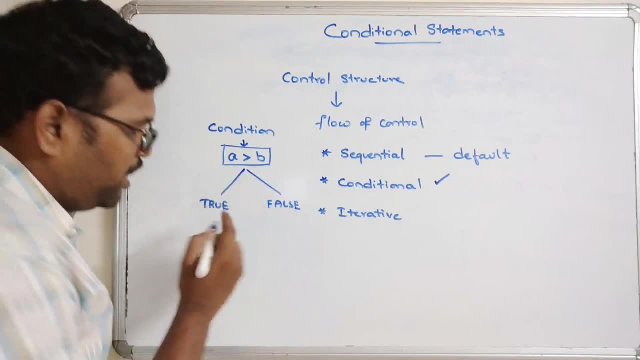 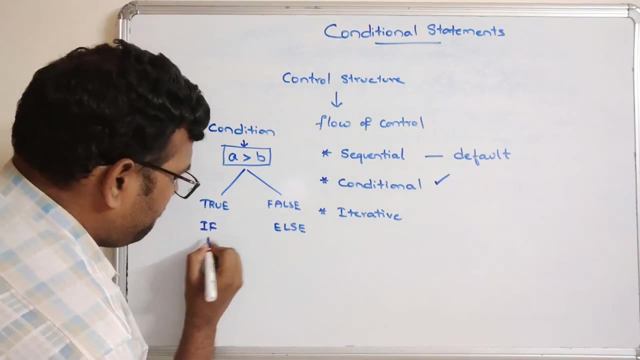 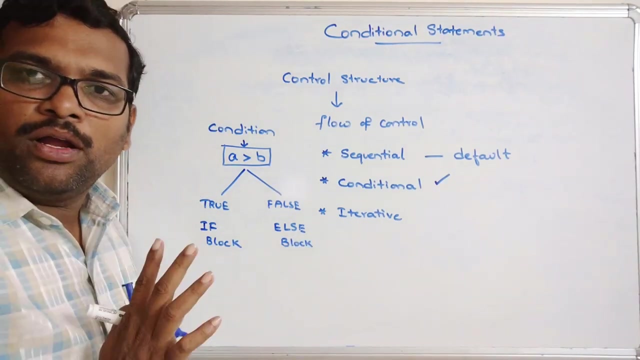 will execute either true block or a false block. so here usually we call it as a if and here we call it as a yes. so if block, if block and block. so if block is a true block and else block is a false block. so here, at a time, based upon the 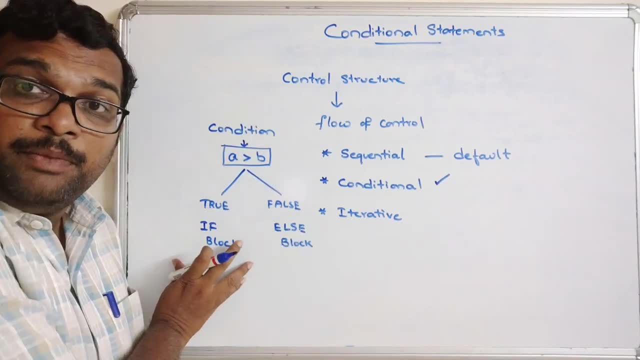 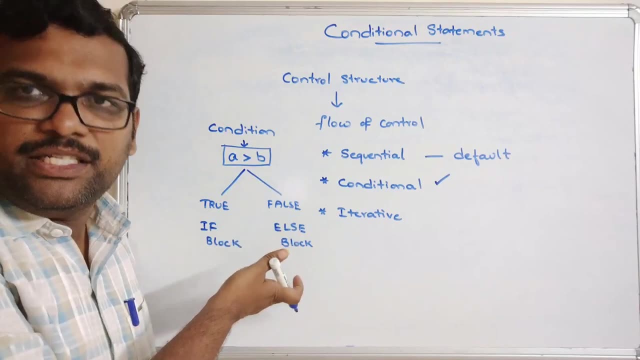 result of the condition, either true block will be get executed. that means, whatever the instructions we are writing under the if block will be get executed, or the instruction written in else block will be get executed. and one more important point is so that we call it as a conditional control. 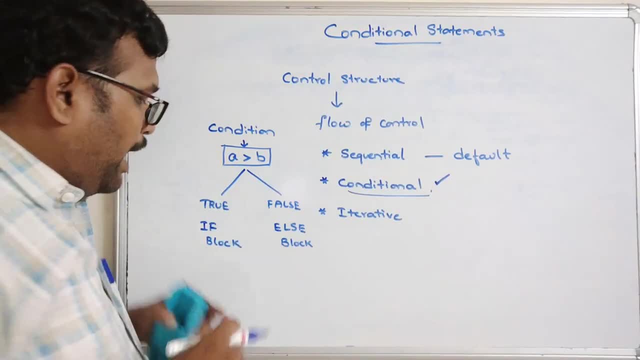 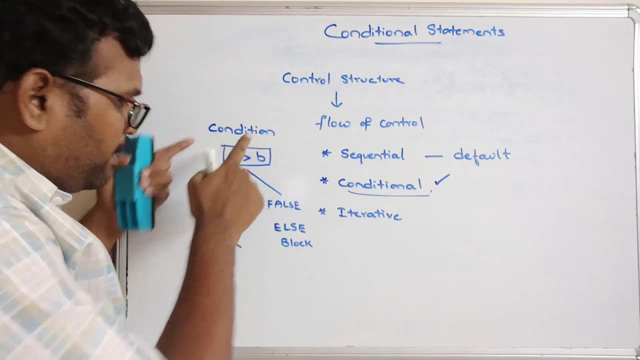 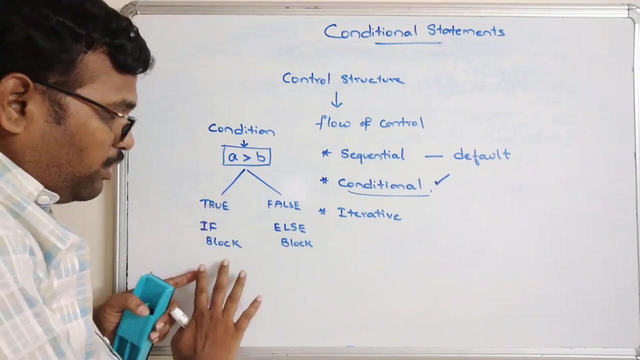 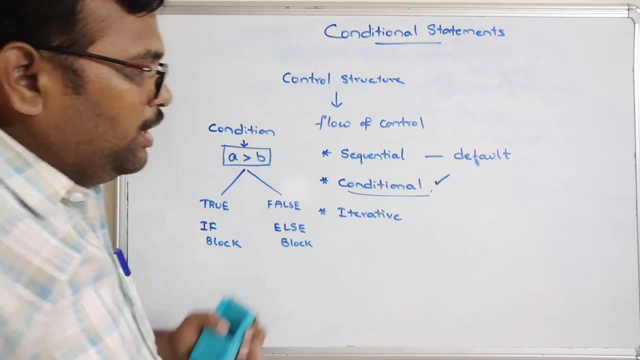 structures, conditional control structures. and here one more point: always the condition should be written in if block only. the condition should be written only in the if block. the condition should not be written on else block okay. so without if block we should not write else, but without else we can write if, because we are writing condition in if block only. so here the 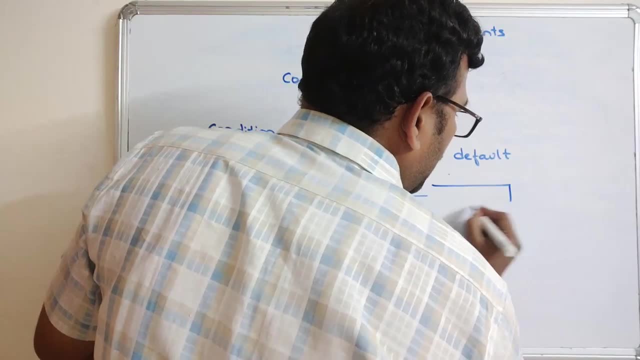 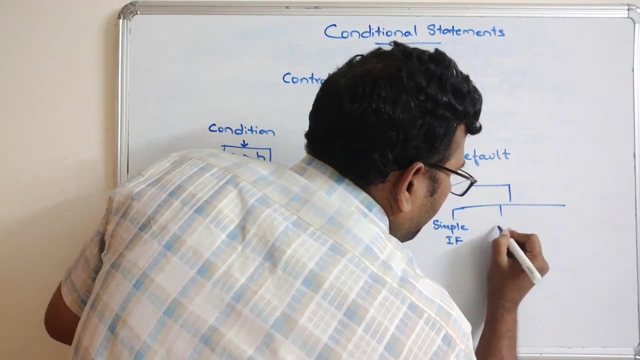 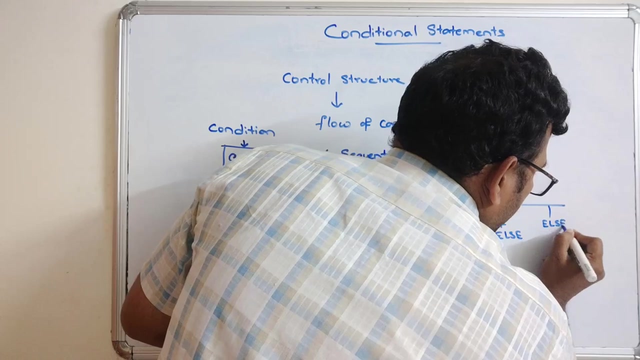 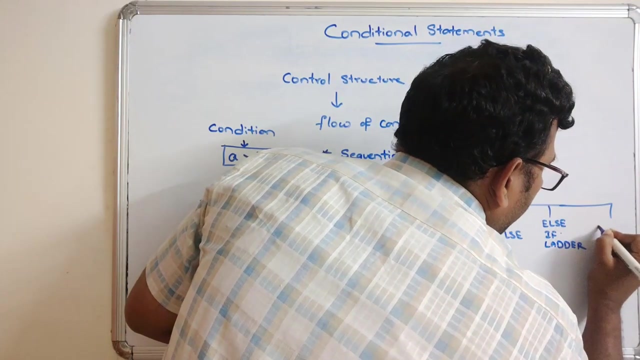 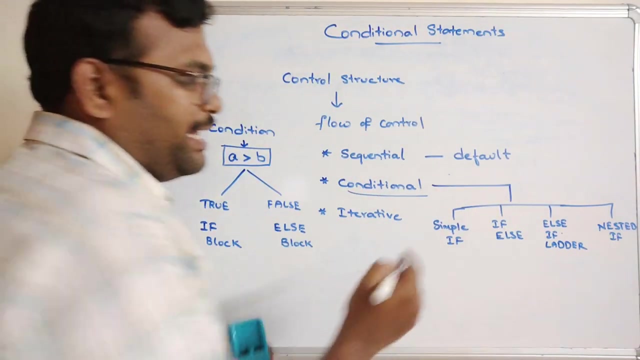 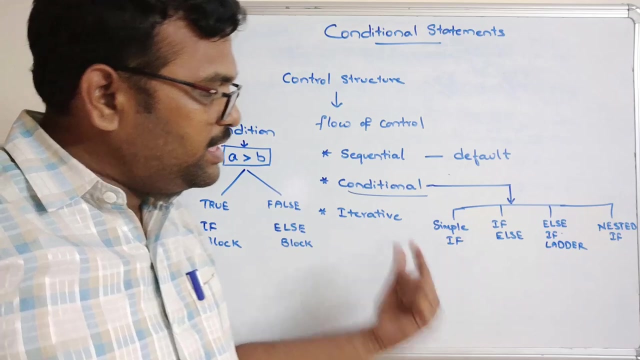 conditional statements are again categorized in different way. the first one is simple: if, if else else, if later nested, if nested, if so. these are the four categories of this control statement. i mean conditional statements. now we'll see the syntax of all these four and then we'll move on. 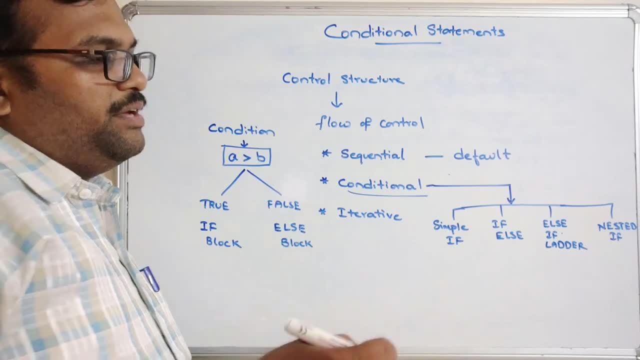 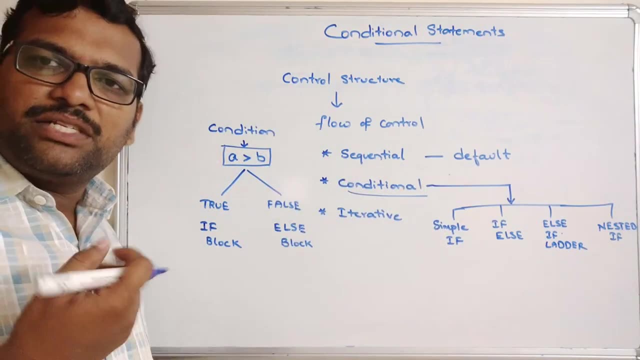 to the r studio and i will show you the example, each and every example, for each and every conditional statement, right? so, other than these four, there is a one more conditional statement that is a switch case, so that we'll discuss later. in today's session. we'll discuss about 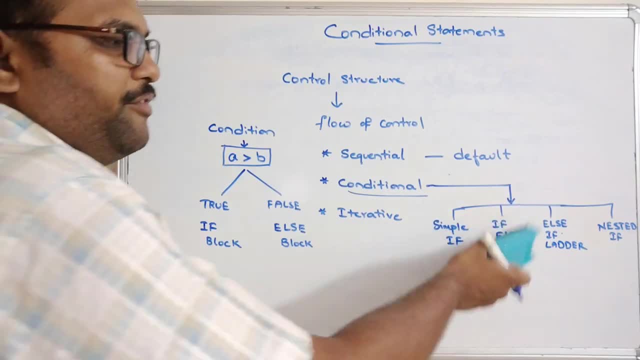 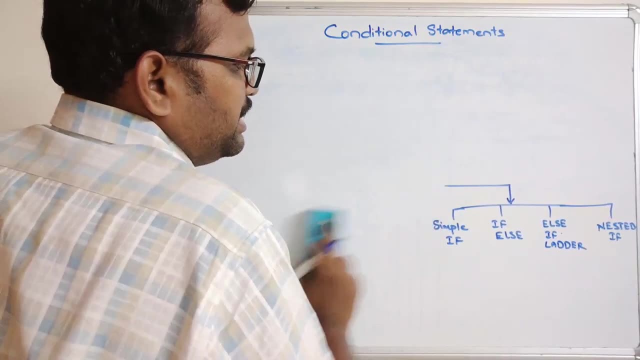 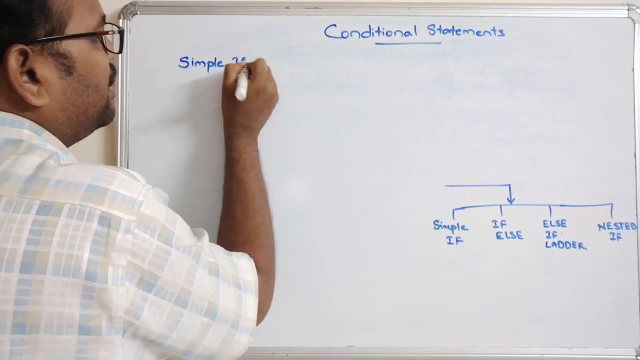 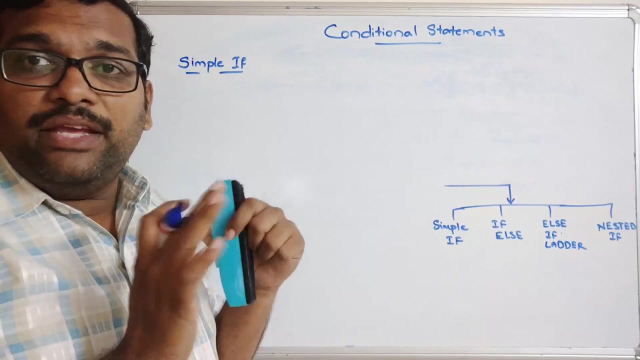 these four conditional control structures: if, if, else else if and nested. so starting with the simple if, simple if. so just now we have said that if is a true block and the condition should be written only at the if block, only right. so without the if we should not write else and without else we can. 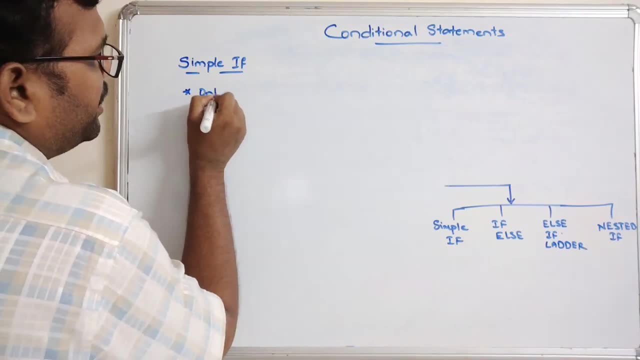 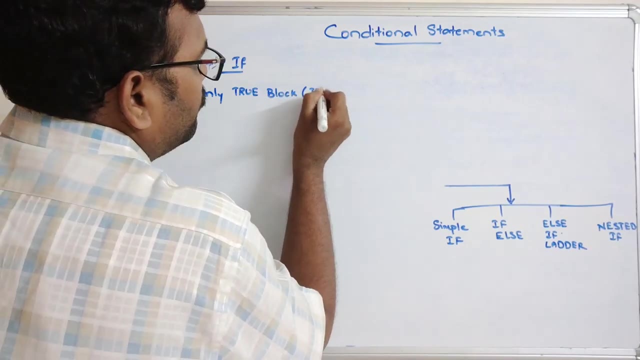 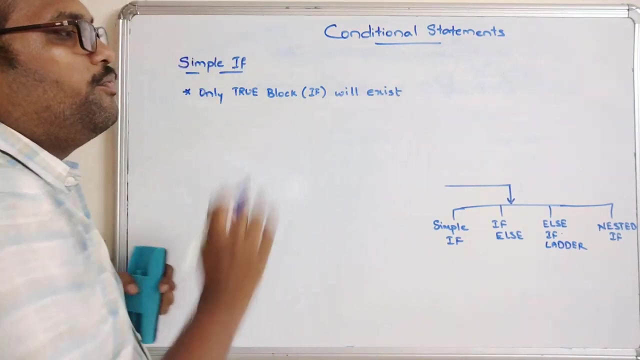 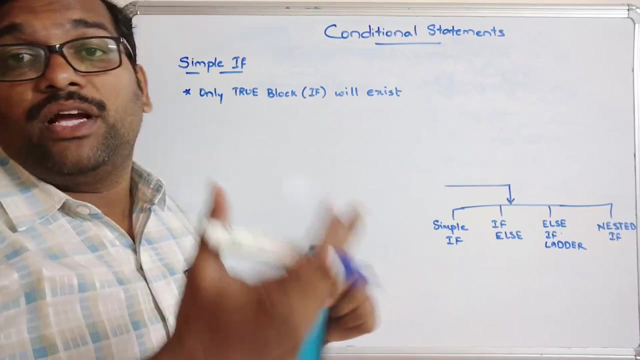 write. if so, here only true block will be there, only true block. true block, that means if block will be, there will exist. So we have to give the instruction to the interpreter, which are to be executed if the condition becomes true as well as if the condition becomes false. 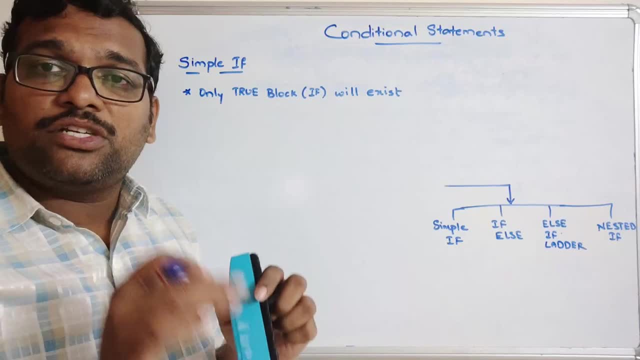 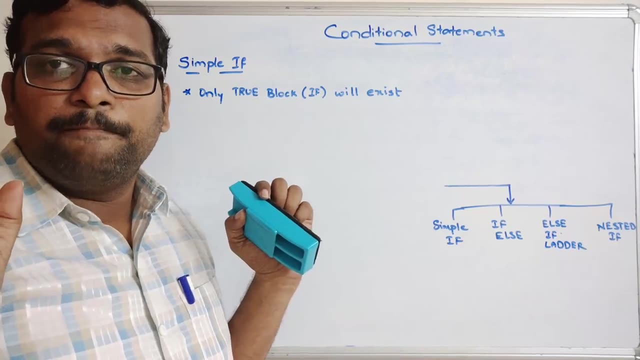 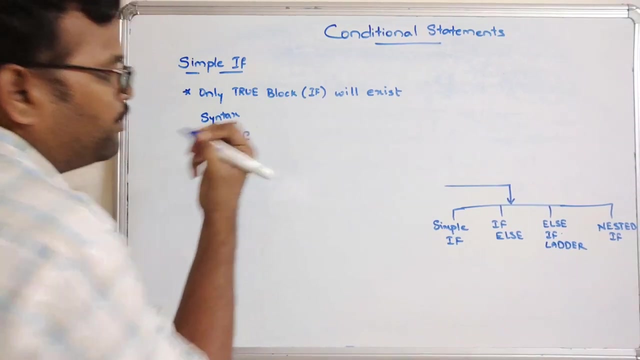 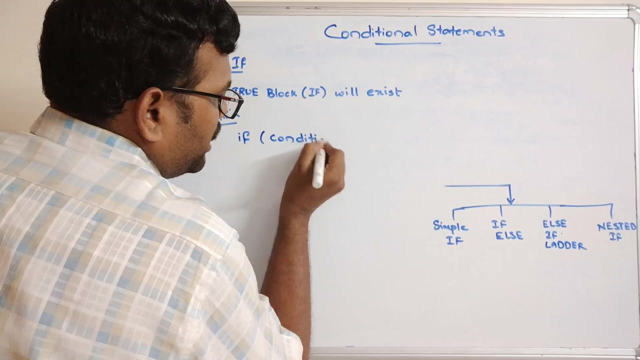 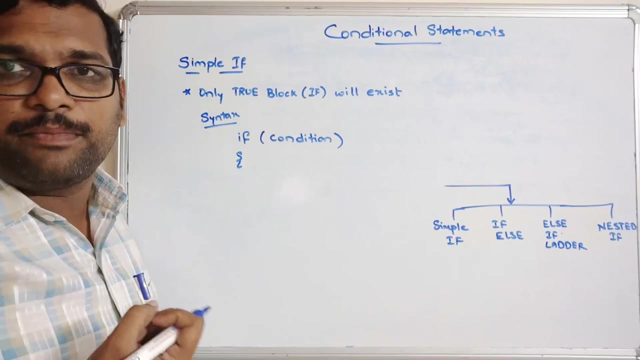 So in this simple if, we are giving the instructions only if the condition becomes true. So we are not giving any kind of instructions if the condition becomes false. So the syntax for this simple if is: if is a keyword, small letters, lowercase letters and parentheses. write down the condition here. write down the condition and open the curly braces in order to represent a multiple statement, that is, a block of statements. 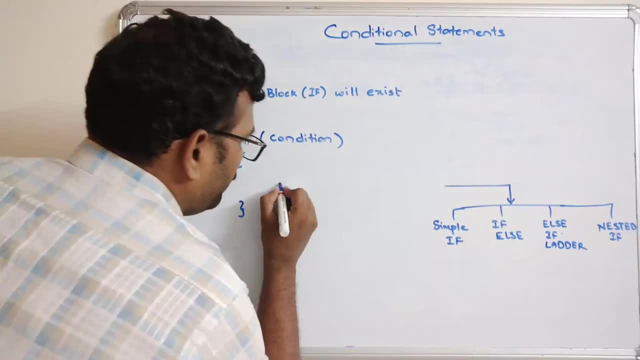 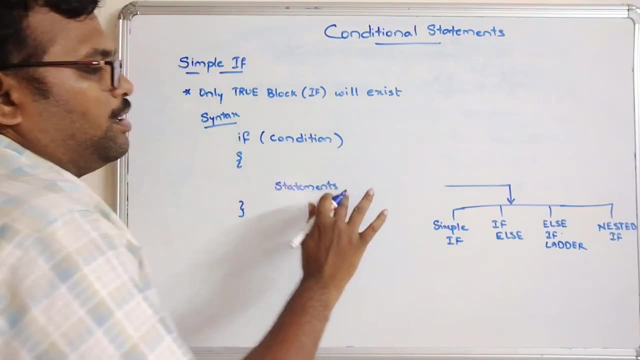 That's it. So this is the syntax, and here we have to write down the statements. So we can write one statement or more than one statement, depends upon our logic, right? This is called a simple. if only true block will be there. 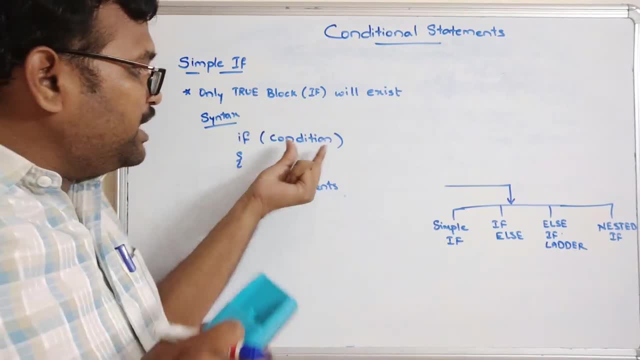 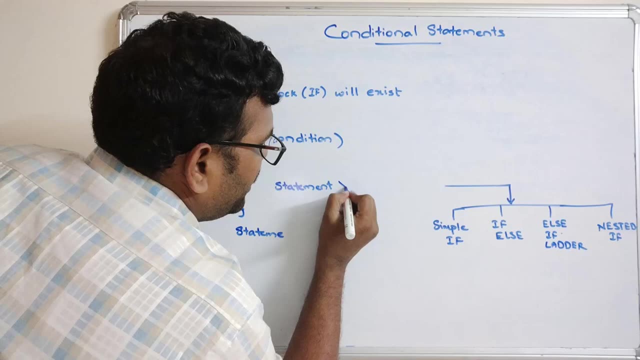 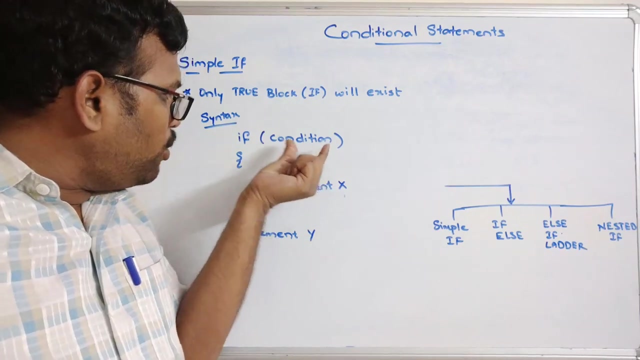 So if the condition becomes true, these statements will be executed. If the condition becomes false and outside the if block statements will be get executed. So we will write here statement x and statement y: okay, If the condition becomes true, then the control will enter into the loop. 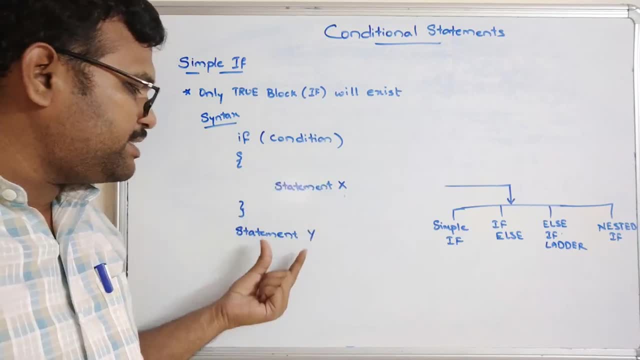 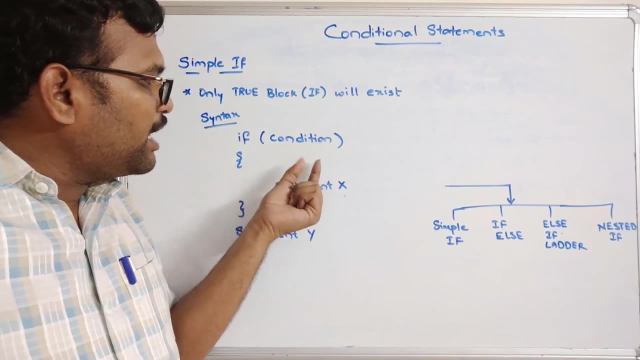 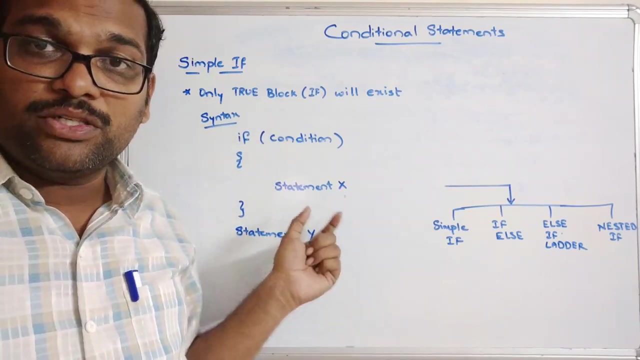 And statement x will be get executed and after that statement y will be get executed, because statement y was written after the if block And if the condition is false, the control never enter into the loop- I mean never enter into the block- and directly the statement y will be get executed because statement y will be the outside the if statement. 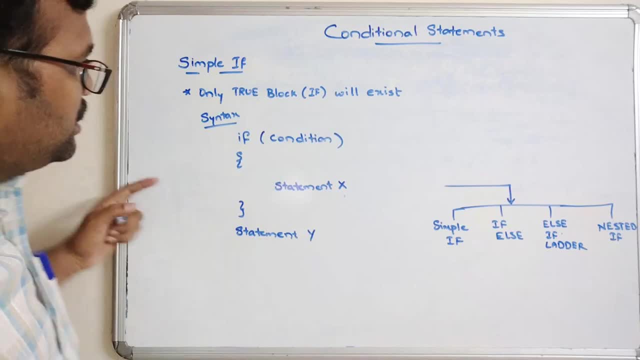 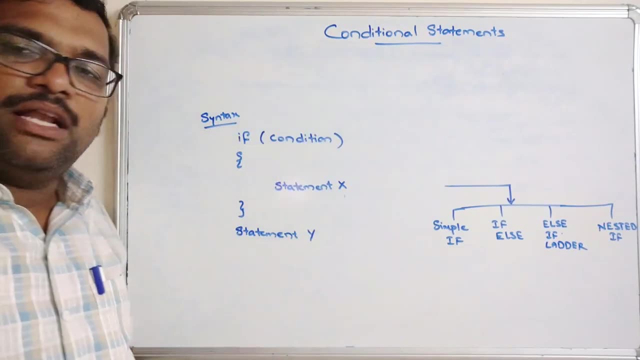 So that will be the sequential execution again, right? So this is a simple if. Now we will write a if else In the if if else the name itself indicates, we have to specify the instructions in both the true block and false block. 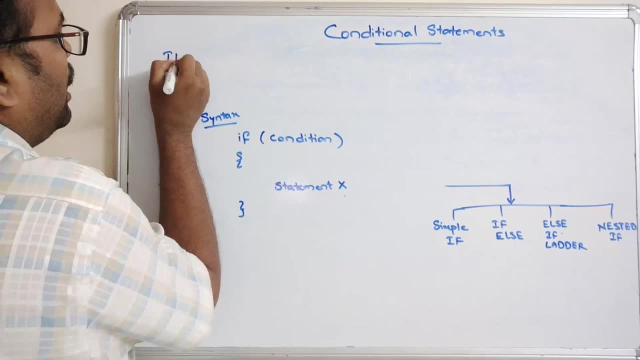 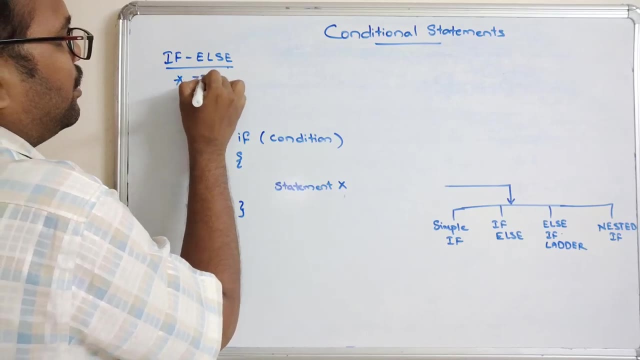 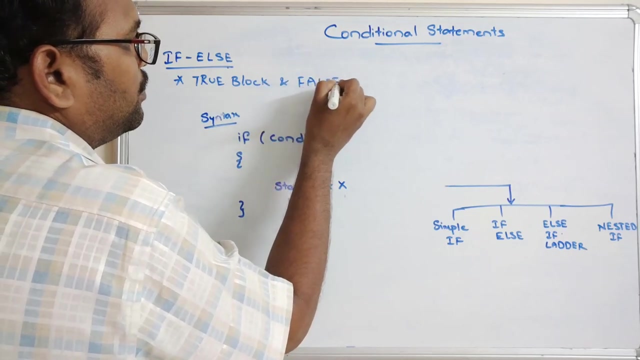 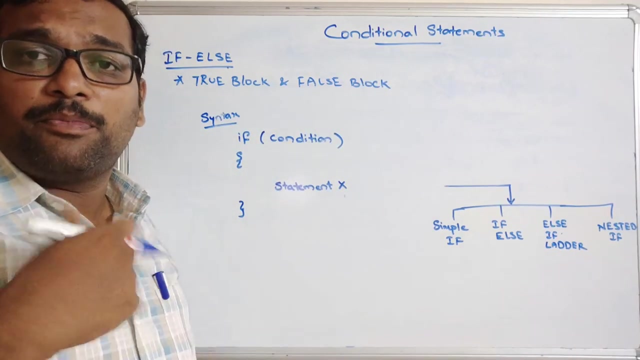 So I will write here, if else, right? So here we have to write true block and false block. So even though we are writing both the blocks, only one block will be get executed. Whether depends upon the result of a condition, right. 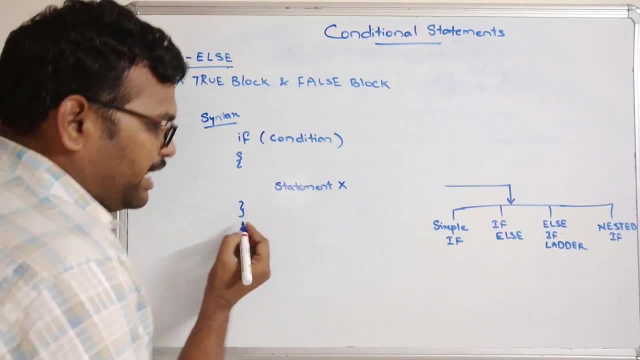 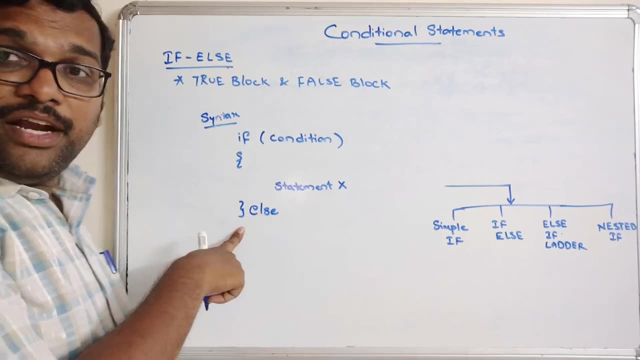 So if here and here one more important thing is, else should be written immediately after the closing braces of if okay, So don't write else outside. okay in the new line, So the closing braces and else should be in the same line. 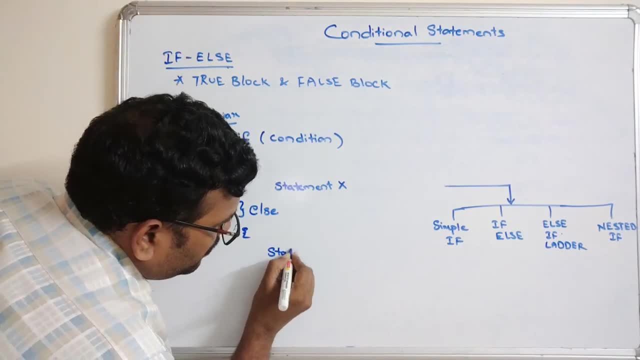 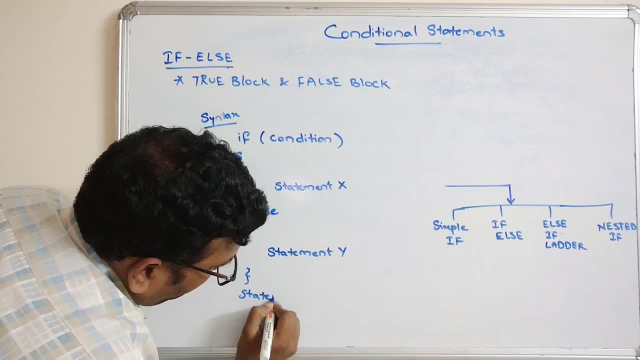 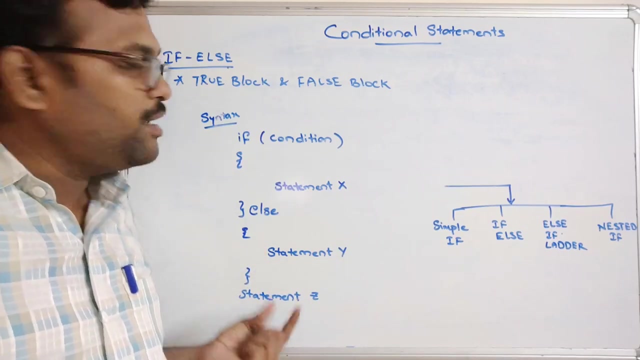 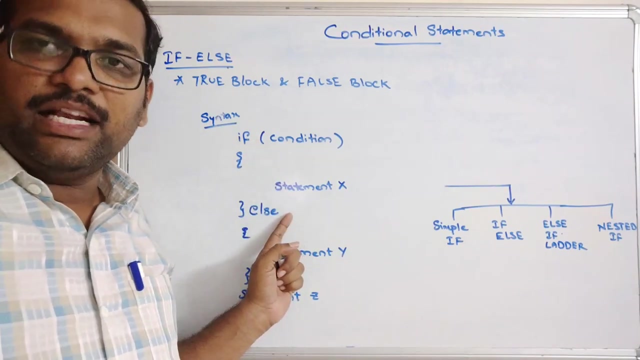 So else open. brace. statement y, statement z. So here this is a syntax for if-else statement. So here always the condition should be written only in the if block right. You should not write the condition on else block. 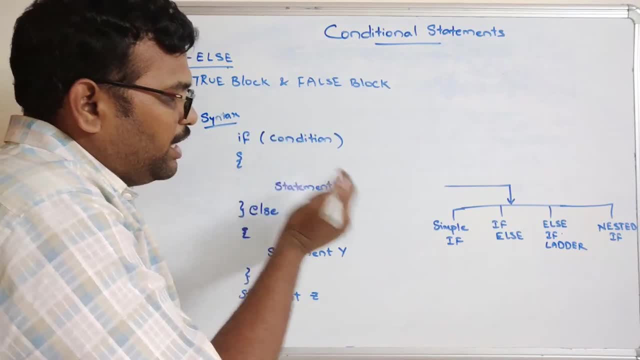 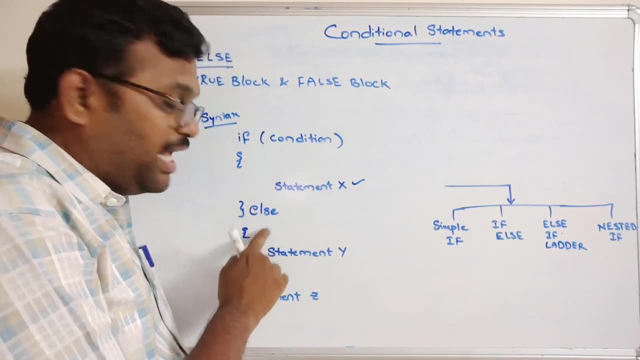 So, based upon the result of a condition, if condition becomes true, statement x will be get executed and immediately statement z will be get executed. So the control never entered into this else, because this is a false block. So if the condition is true, the true block will be executed. 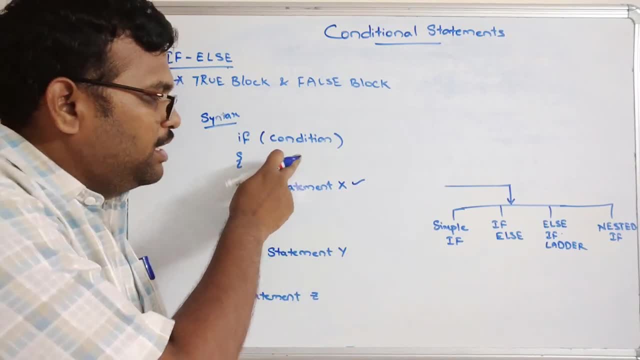 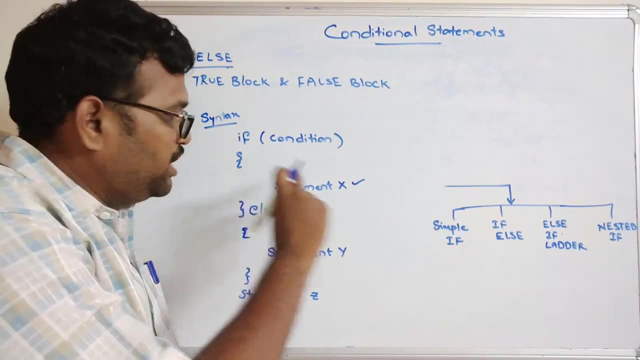 and the false block will be ignored. And if the condition becomes false, directly the control enter into the else block. The control never enter into the if block because if is a true, So this block of statements will be executed only if the condition becomes true. 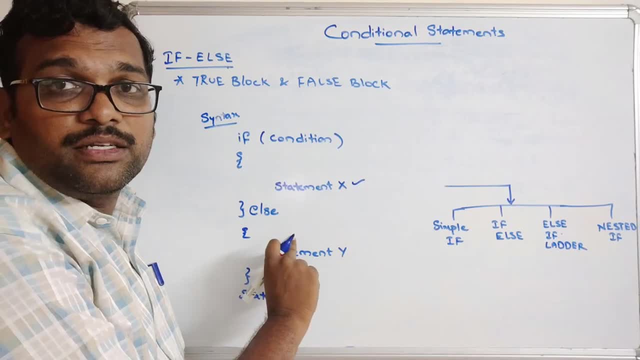 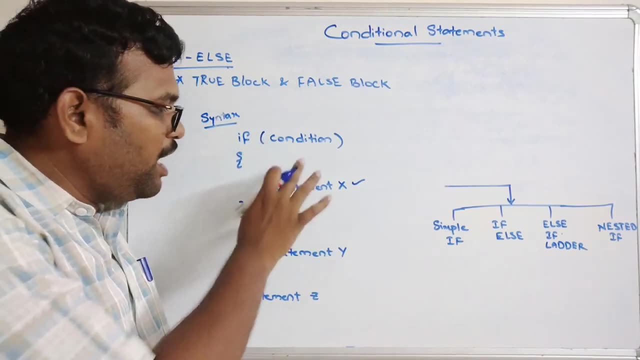 And this block of statements will be executed only if the condition becomes false Right. So only one block of statement will be get executed based upon the result of the condition, And immediately after that the statement z will be executed commonly, because that was written after the if-else block. 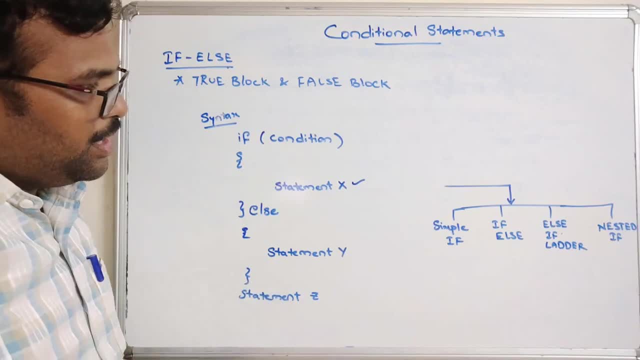 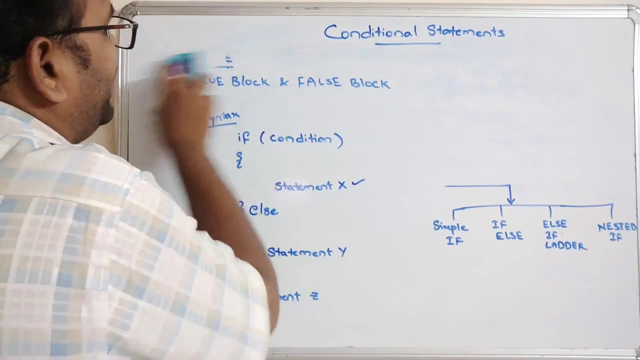 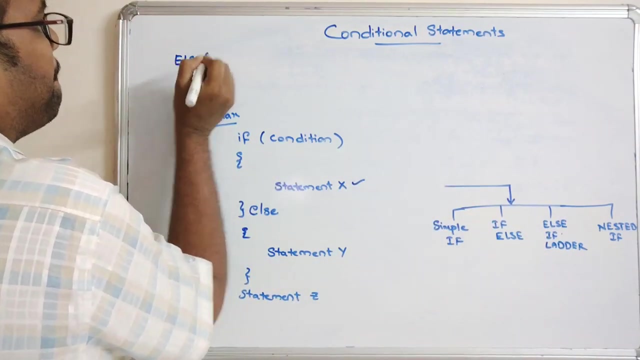 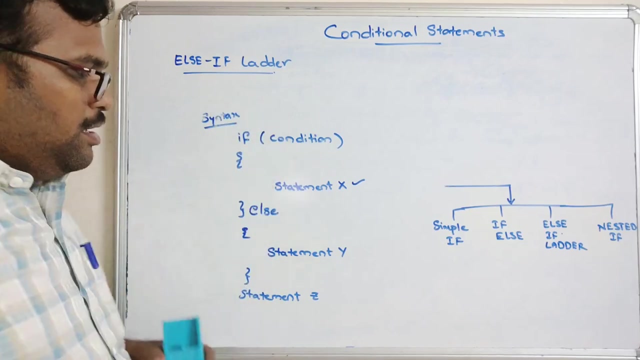 Right, So hope you understood this one. So, example, I will show you the implementation part in the laptop. Okay, Now we will move on with the next one, that is, else-if ladder, Else-if ladder. So here, if we want to check multiple conditions, 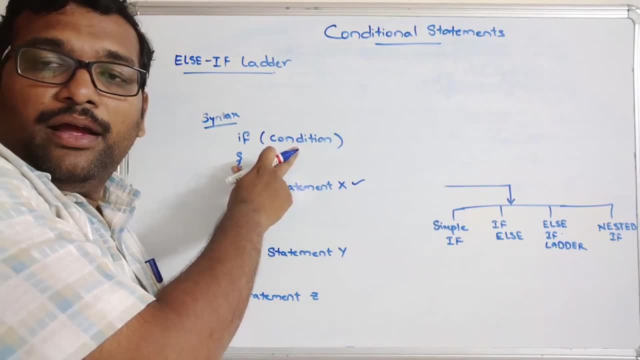 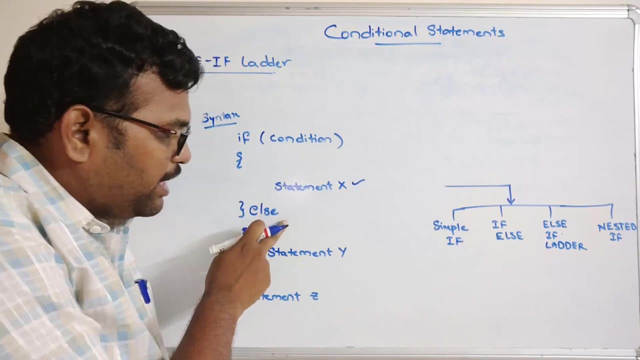 okay if one condition is already verified and based upon the result of the condition again. if you want to check one more condition, then we have. we should not write the condition in the else, right? So that's why we have to include once again if and we can write the condition. 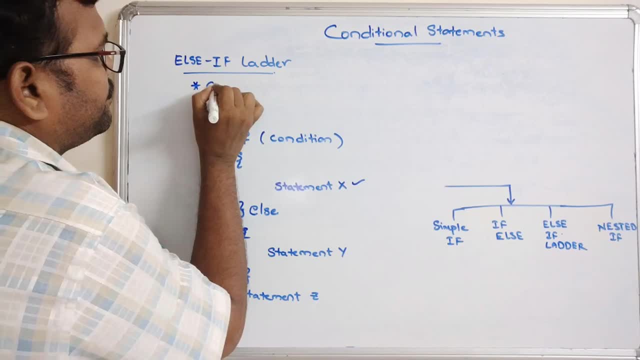 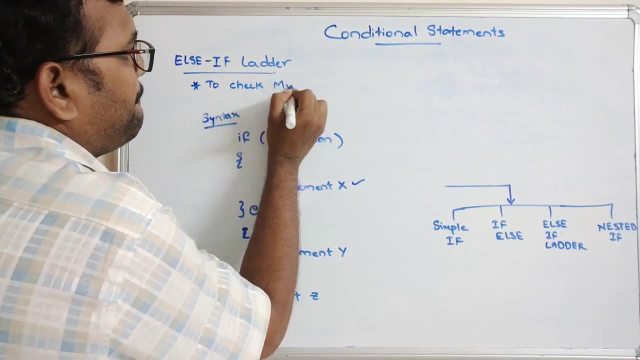 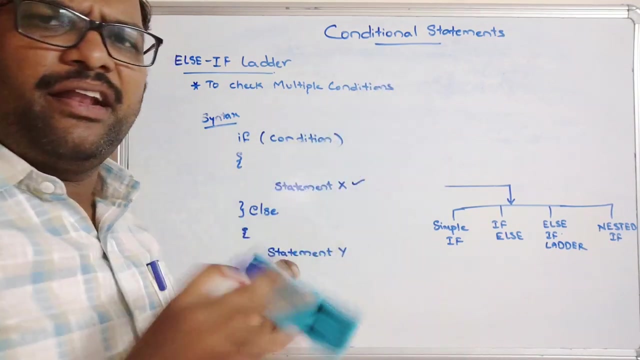 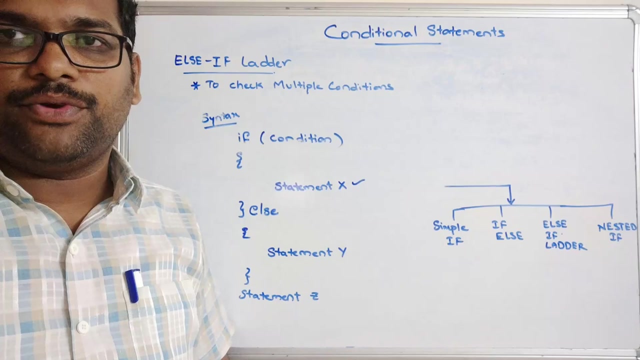 So in order to check multiple conditions, To check Multiple conditions, So n number of conditions can be written here, Any number of conditions. So, even though the number of conditions have been written, only one block will be get executed. 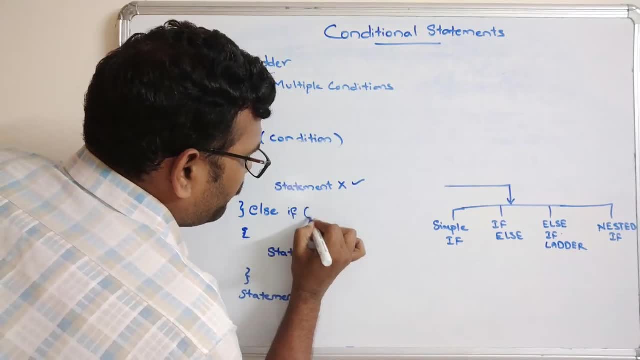 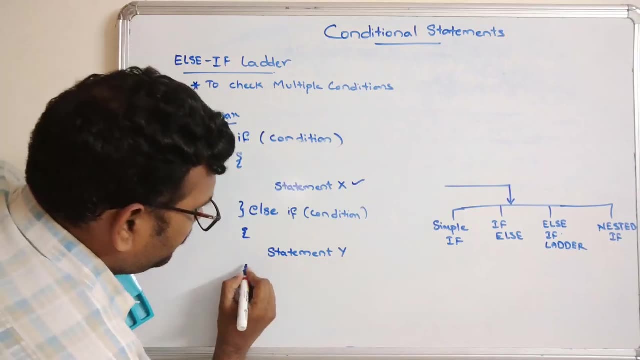 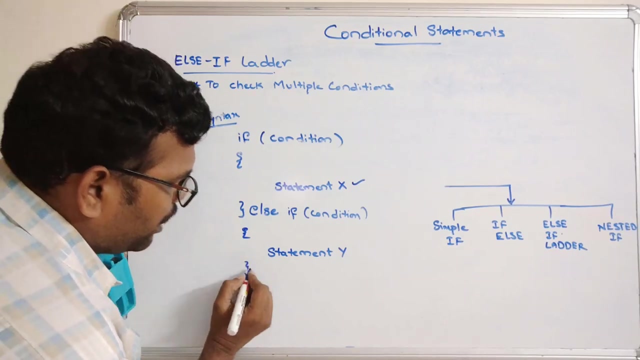 For example, see else, and again here we have to write one more condition If you want to check it Right, And after that, simply you can write the else part and you can repeat the same thing multiple times. If you want to write multiple statements, you can repeat it multiple times. 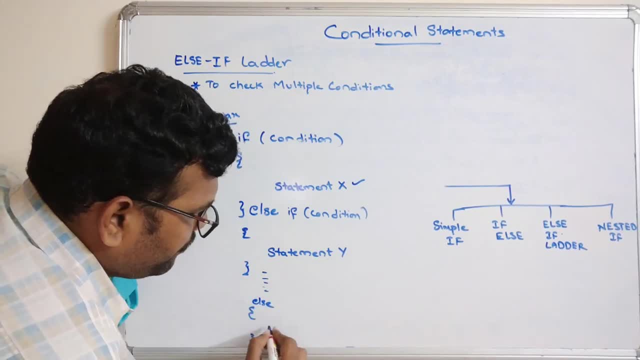 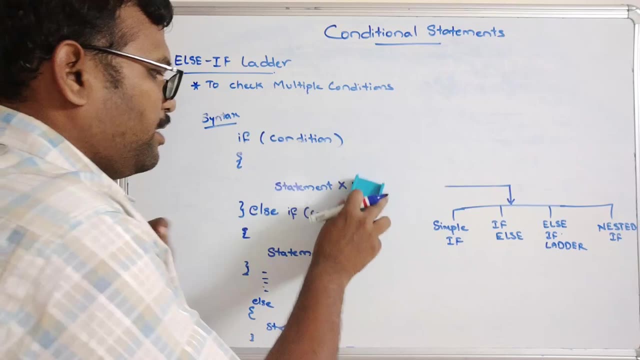 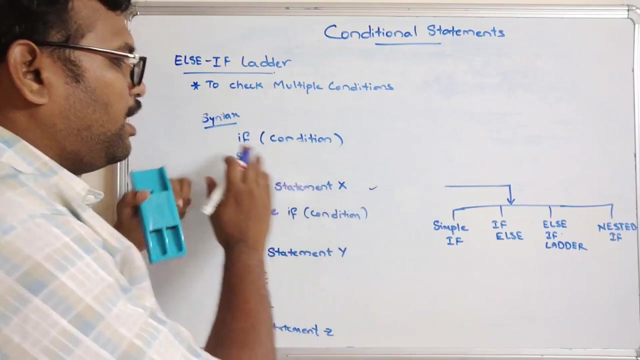 And finally, the else part can be written here: Statement check. So first, this condition will be verified and based upon this condition. if this condition is true, this will be executed and automatically the control will never enter into any other condition. 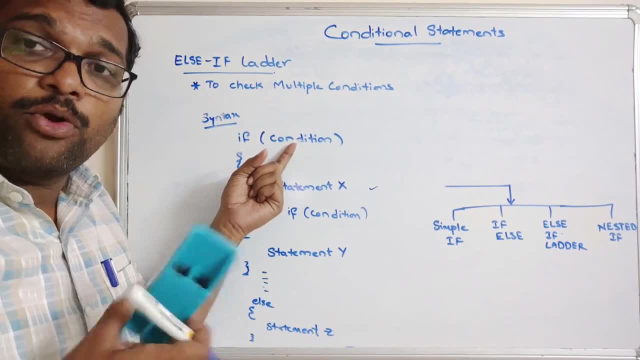 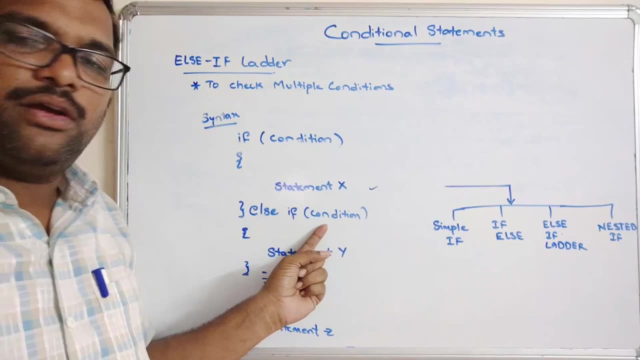 If the condition becomes false and if you want to check one more condition, then simply it moves to the next condition. And here also, if the condition is false, it will move to the next condition. So if the condition is true, then it will stop. 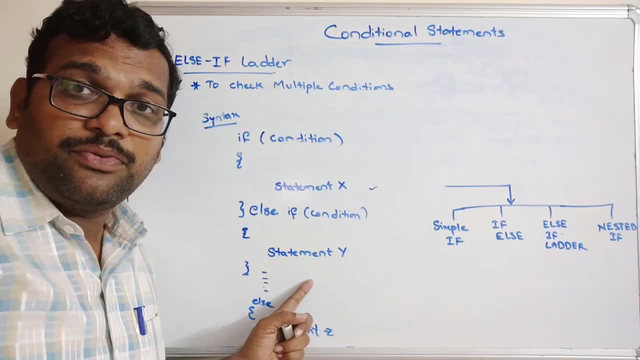 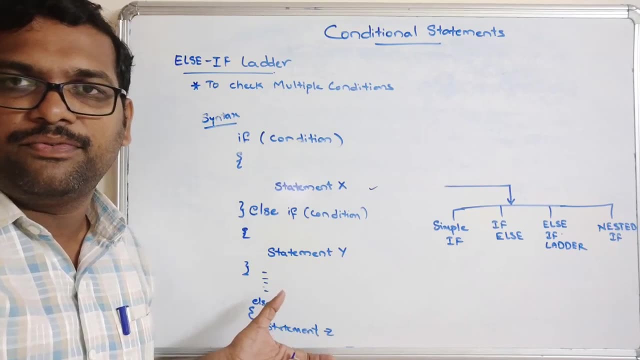 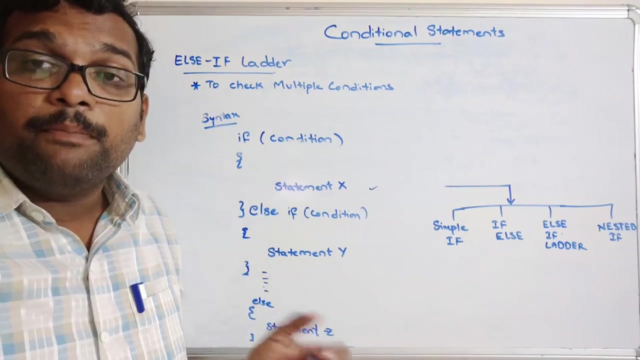 It will enter into that particular block and it will stop executing the complete else if ladder. So here we can write multiple number of conditions, So hundred conditions also we can write, but only one block of statement will be executed. So if the condition is true, then it will stop executing the complete, else, if ladder. 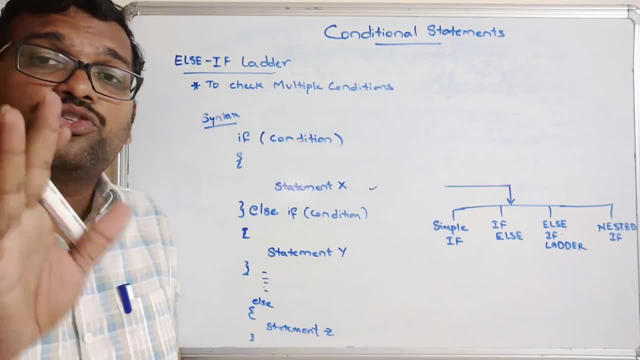 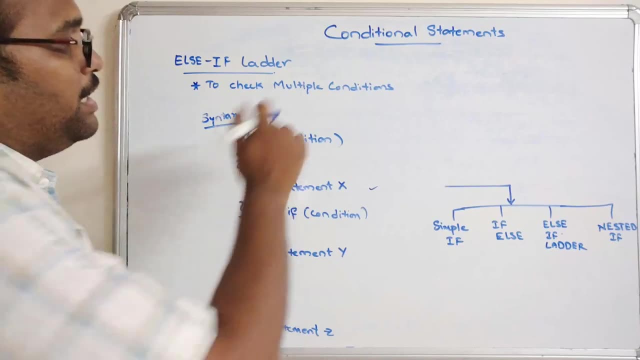 And this block of statement will be executed. So whenever the condition becomes true, then only that will be executed. Otherwise the else part will be get executed. OK, so in order to check multiple conditions, we are going to use this. else, if ladder 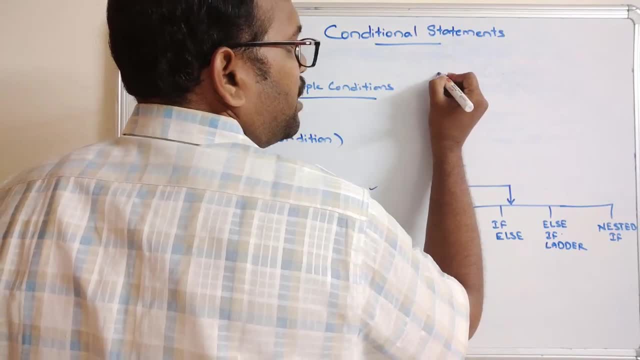 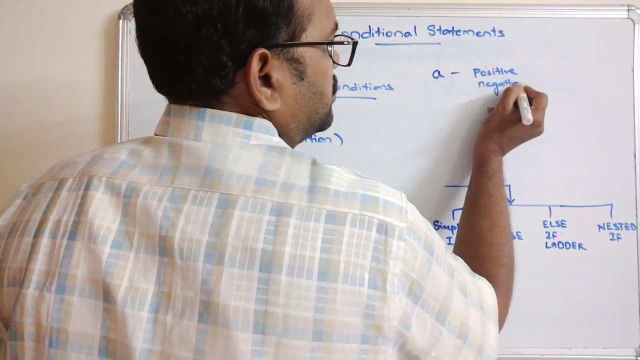 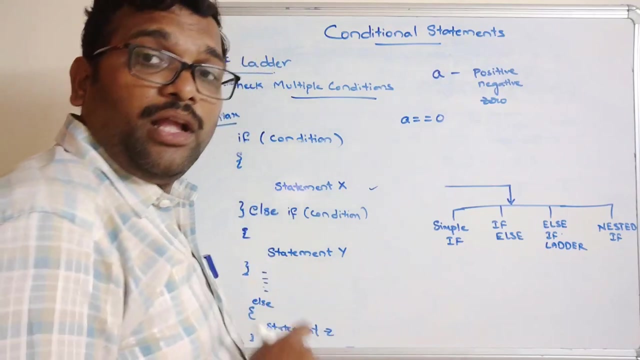 For example- let us take some. We need to check a number: is a positive, Negative, Or a zero Or a zero? So first we can check: a is equal to is equal to zero. if it is true, then we can simply say that the given number is zero. 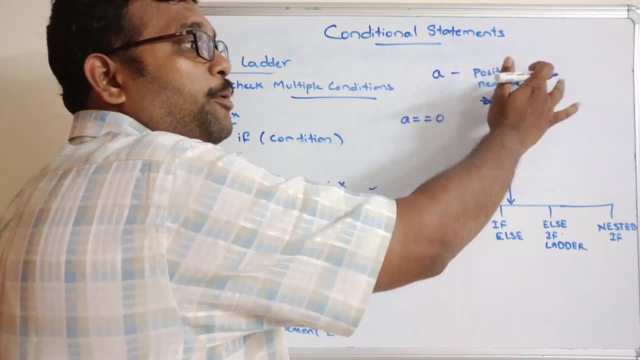 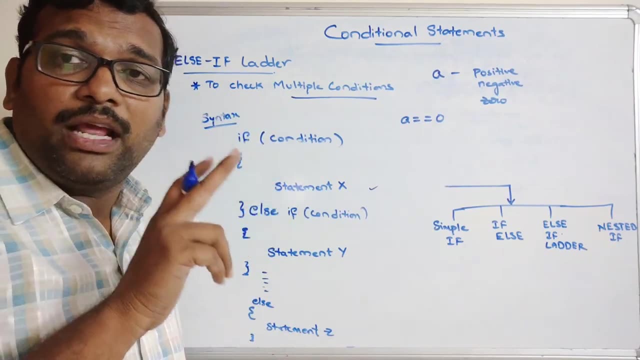 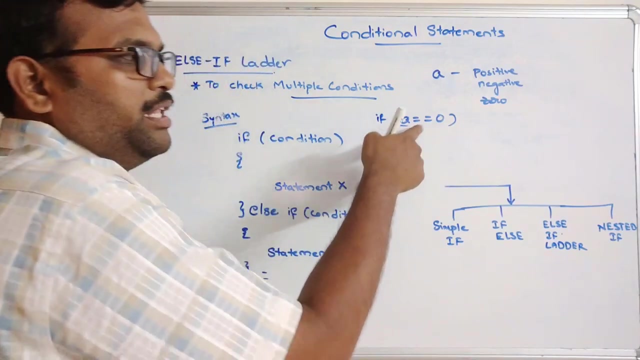 if it is not zero, we have to check whether it is a positive or a negative number. okay, again we can have. we are having a two things: it can be a positive number or it can be a negative number. so once again we can write. so this is a if statement and else means nothing but the. 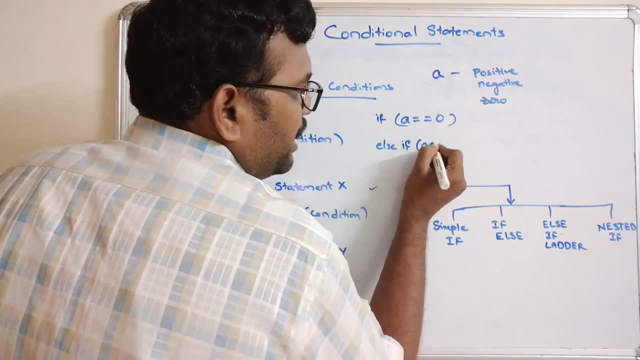 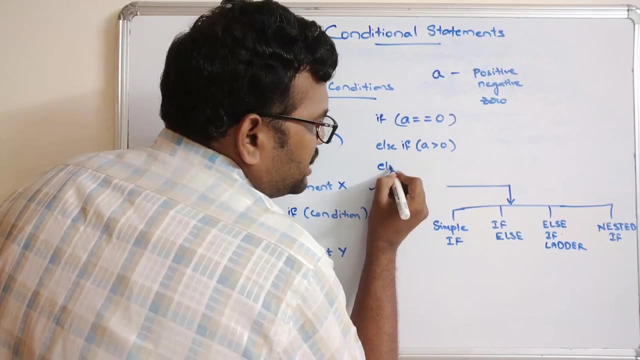 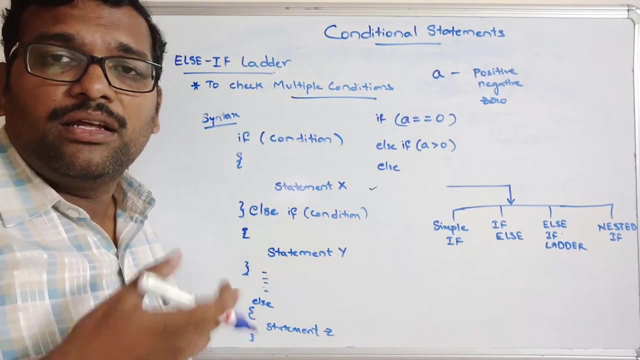 condition becomes false. again we have to check condition. else, if a greater than zero, then simply we can say it's a positive number. and if both the conditions are false, simply we can say else, simply it's a negative number. if, if a number is not a zero and not a positive, obviously the number 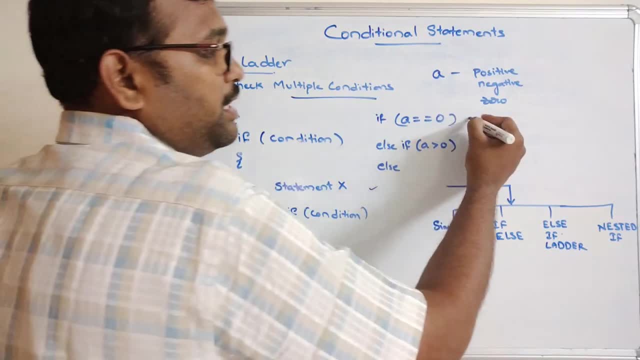 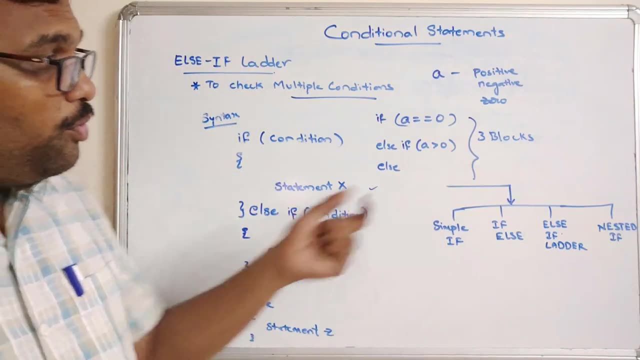 will be a negative number. so here we are writing the three blocks, three blocks of statements. right, here we are writing three blocks of statements, but the only one block of statement will be get executed. okay, not all the three blocks will be get executed, only one block of statement is. 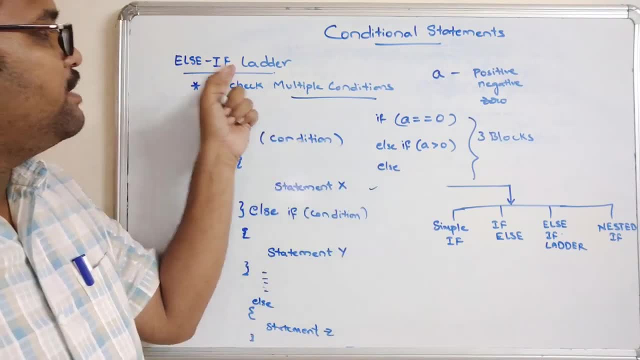 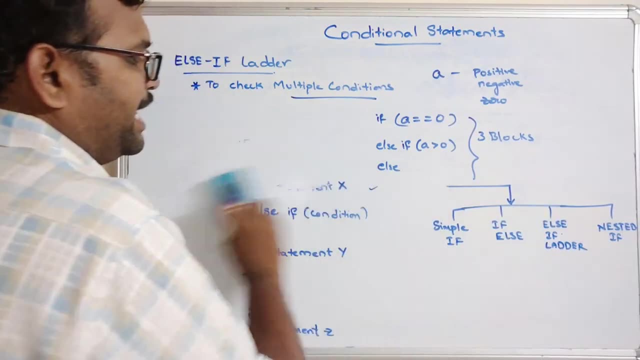 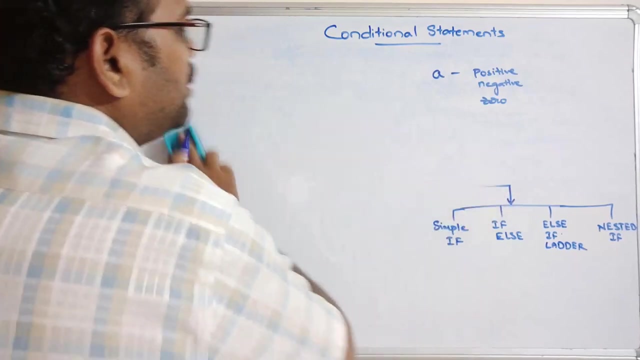 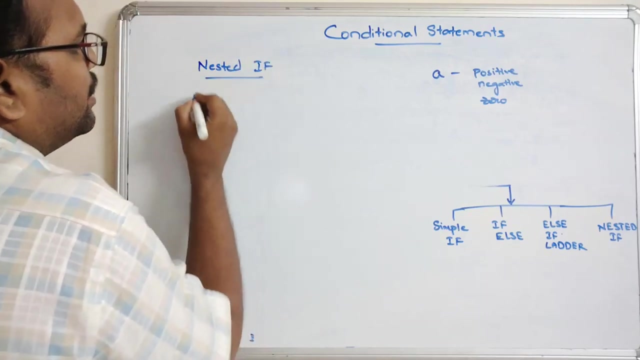 being executed. so if we write three blocks of statements, then only one block of statement executed. so this is called the else- if layer, so multiple conditions can be written here right. next last one is a nested if nested if the name itself indicates we can write the if block inside another if block. so let us write nested, if right, so we can write if. 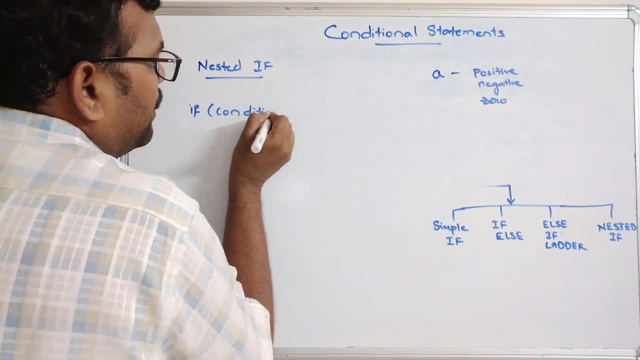 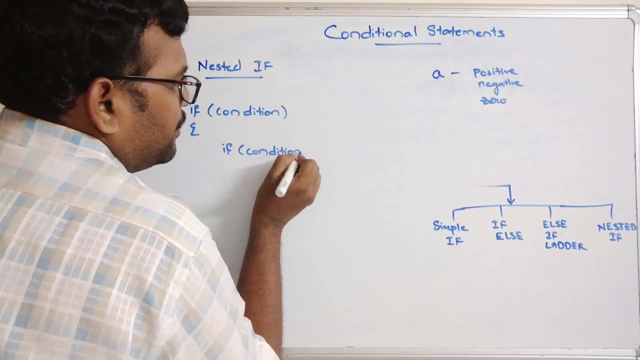 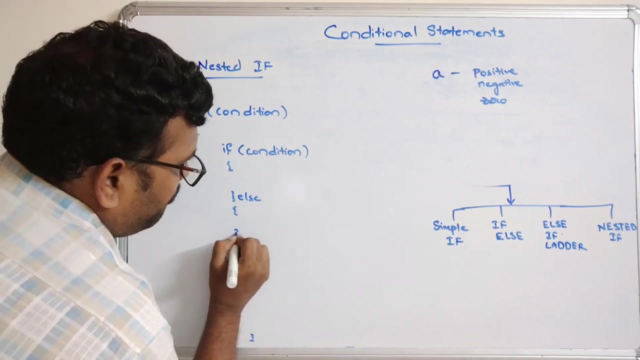 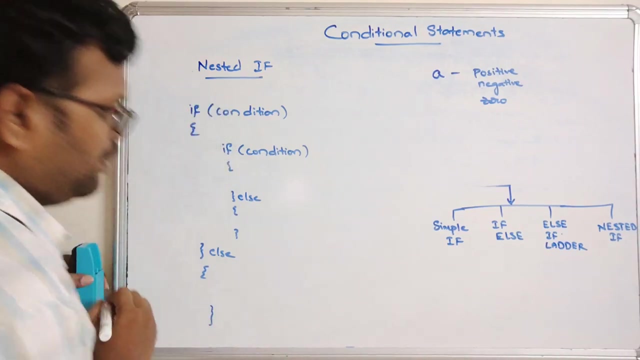 and condition, if condition. and if the condition is true, again we can write one more condition here, we can check one more condition here. so here we can write else and here we can write else, right? so like that, inside the if condition, once again we can write this: if: 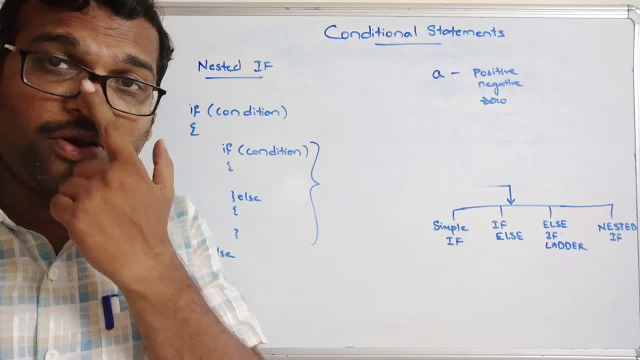 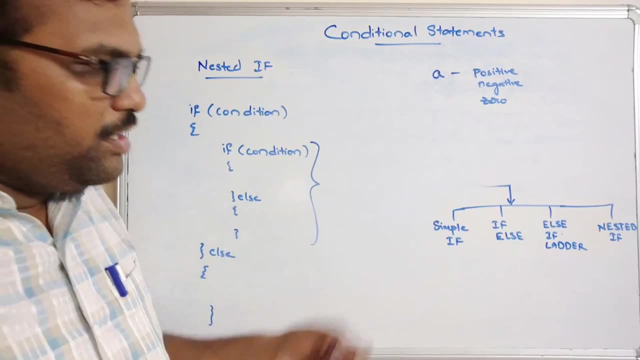 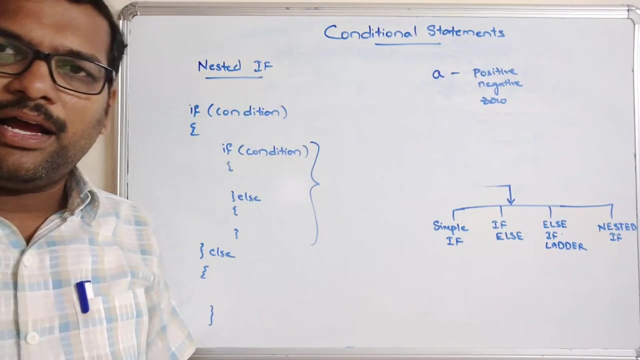 else? condition depends upon our logic. ok, depends upon our logic, so do not worry, I will explain everything by implementing with a simple example. right, so we will see all the four conditional statements simple: if, if else, else, if, layer nested, if. with a simple example, I will execute for each. 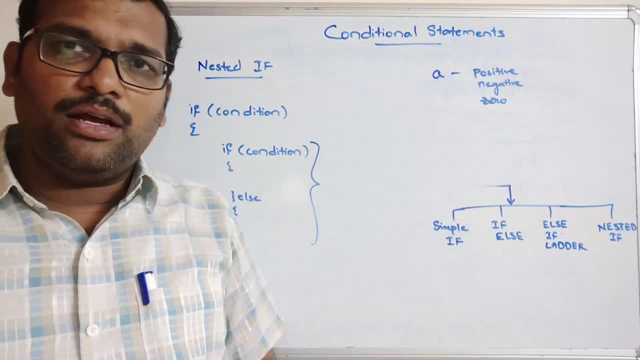 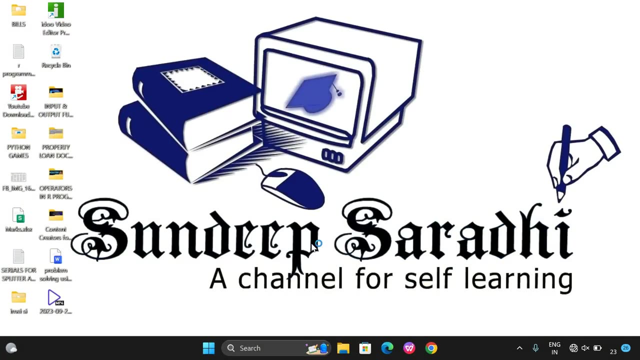 and every conditional statement, right. so let us move on to the computer so that I will execute everything on the R studio. right, let us move on. ok, hello friends. so just now we have seen the syntax of conditional statements: simple if and if else. now we will see the implementation part. so let me open the R studio and here 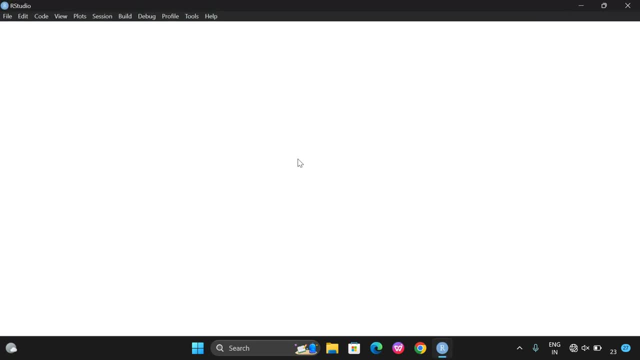 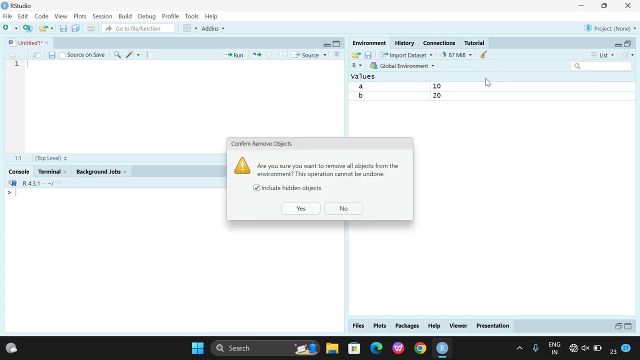 we will see a simple example which you can understand, the working of simple if and if else statements. so before that I will clear everything. now let us write here. first let us take an example for a simple if so, let us take one variable, so n is equal to as dot integer and directly we are converting. 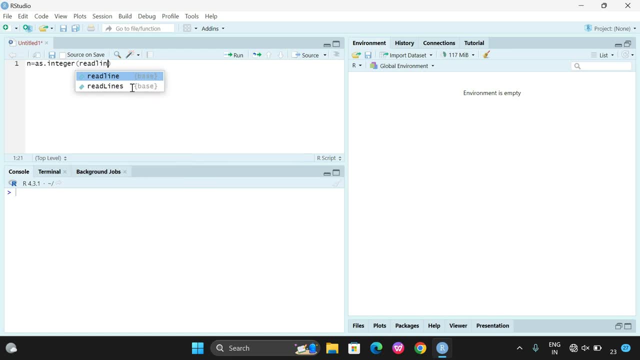 it into integer and we are applying the read line function. so enter value of n so we will check whether the given value is a either positive or a negative right. so you can see we can write an if and followed by the condition here we need to write if. 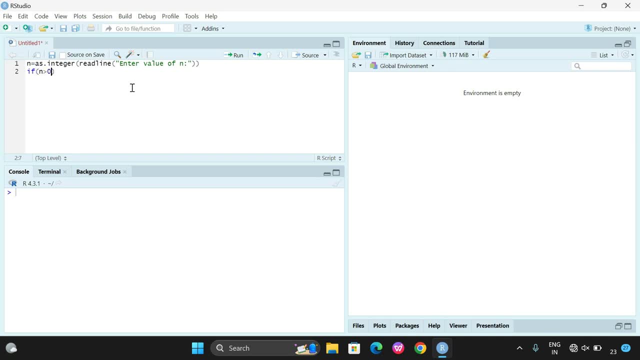 so if n greater than zero, so if n greater than zero. n greater than zero is a condition which gives the boolean result either true or false. if the condition becomes true, then the true block will be get executed. so here what we have to print. so, cat, which is a output. 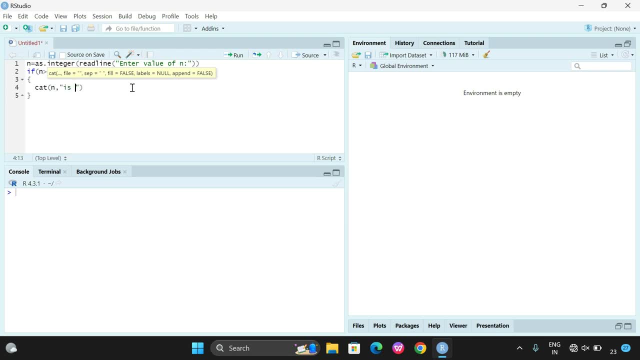 function. so n is positive number right here. just I am giving only if condition. so if n is positive, So we are not writing any else condition. so else will be the false block, and this is an example for simple if so we need not write the else part. that means a false statements. 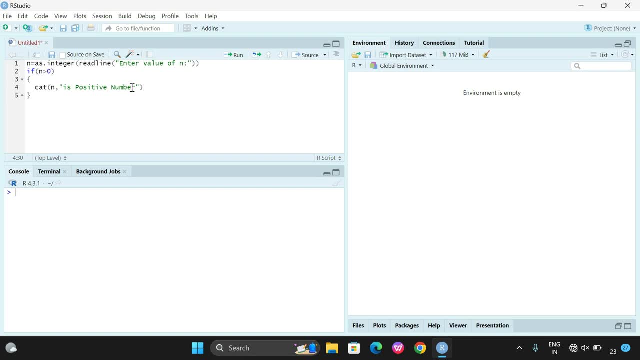 so only we can write only the true block, we can ignore the else block. right, so simply we can execute this one, so it will prompt for n if we give some value which is greater than zero, so we will get the result as a ten is a positive number. you can observe here: 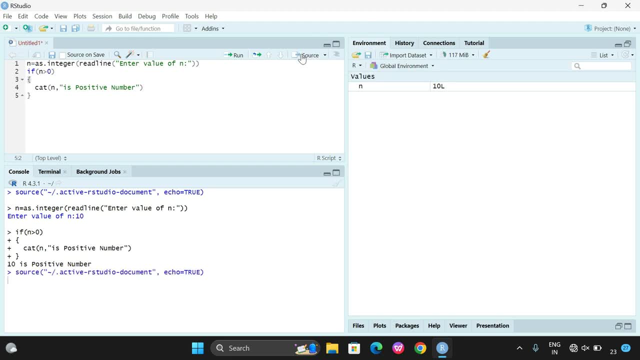 and if again, just execute if you give the n value as a minus one, so nothing happens, because we are not giving the instructions what to be get executed if the condition becomes false. because this is a simple if condition, ok, simple if condition. so here we are supposed. 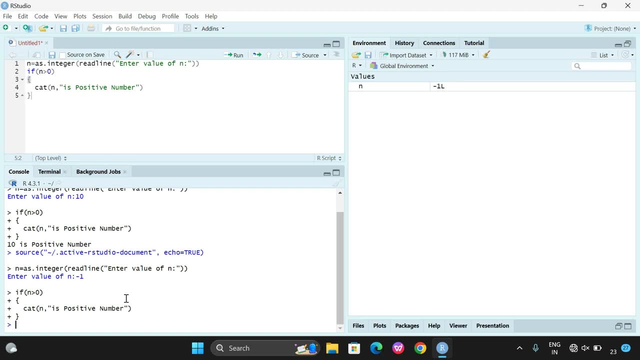 to give only the true block statements. that means the statements or instructions which are being executed only if the condition becomes true, Right. so this is a simple example, for if else? now we will see one more thing else also. that means we have to pass the instructions which are being executed if the condition 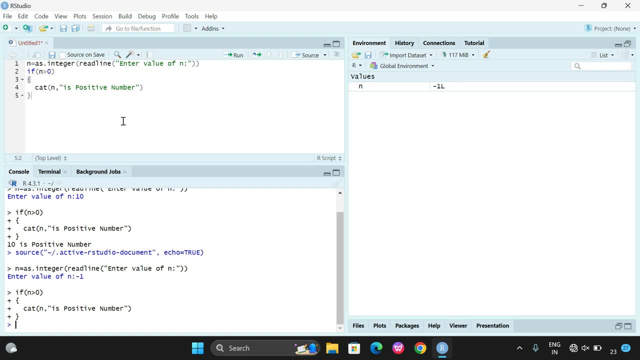 becomes false. now we have seen the condition becomes true. and if the condition becomes false we have to write everything in else part, right? so remember, else should be written immediately after closing of the if condition block, right now. so here again I will write: here n is negative number, right, so let us execute. here n I will give minus ten, so we. 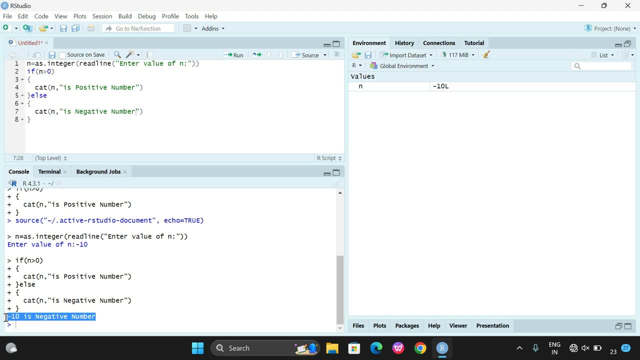 get. minus ten is a negative number. minus ten is a negative number, right? see, one thing you have to remember, so else should be written immediately after the if closing braces. so if you go here, so you will get an error, see error in source. unexpected, else, right? so 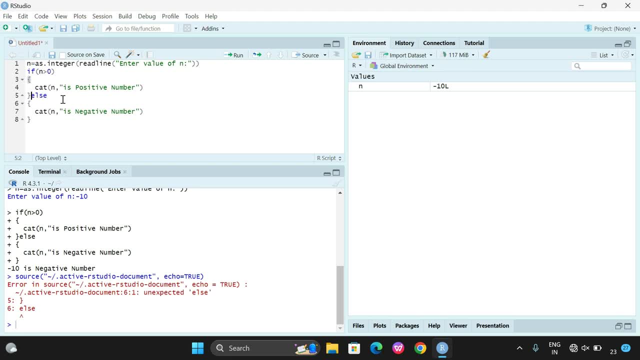 we have to write the else immediately in the same line after the closing brace of if condition. right? so this is an example of if else, if else, right now. else if letter else if letter, right now. else if letter, else if letter. So here we are. we are checking only for positive or negative. then what about if you, if you? 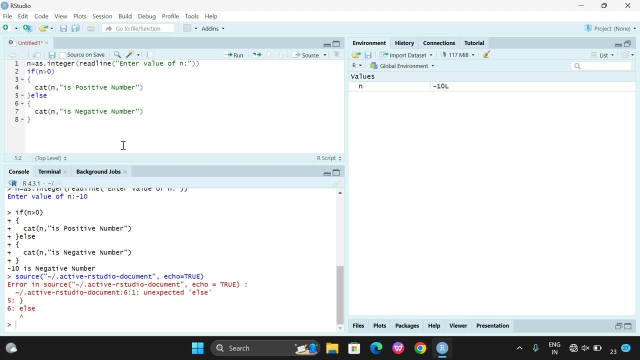 if you give the input as zero? if you give the input as zero, what happens? so if you execute the same thing and if you give the input as zero, we will get. it is a negative number, but it is a false right. so here, in this case, we need to check one more condition, right one? 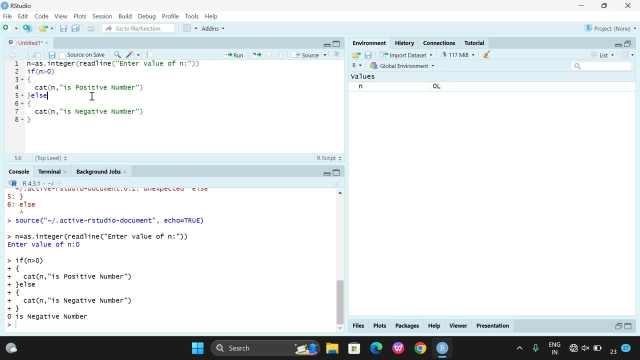 more condition, so where we have to write down the particular condition, so inside the else start again. if so, one thing you have to remember as a condition, right? so if you have to write down the particular condition, right? so if you have to remember as a condition, right. 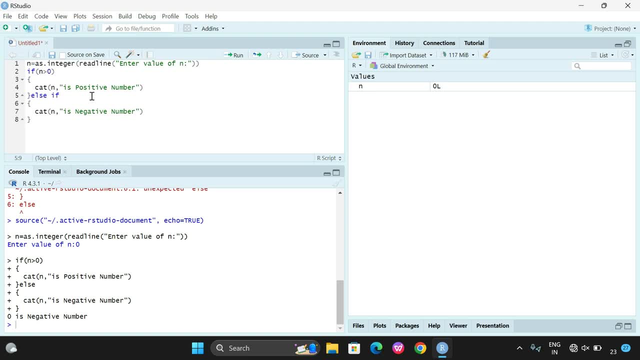 so if you have to remember as a help side in the class, so the condition should be written only in the true block, not in the else block. so here we need to check three conditions. okay, one is: given number is greater than zero. given number is less than zero given number. 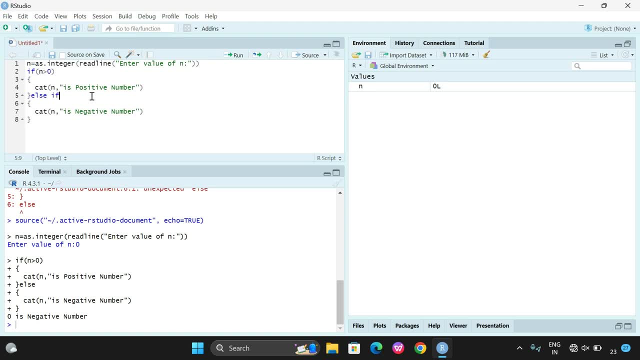 is equal to zero. so we need to check three conditions right, so if the given number is a greater than zero, we will get the result as positive number. again, if it is false, we have to check two more conditions, that is, whether n is less than 0 or n is equal to 0. If n is less than 0, again we have to get a. 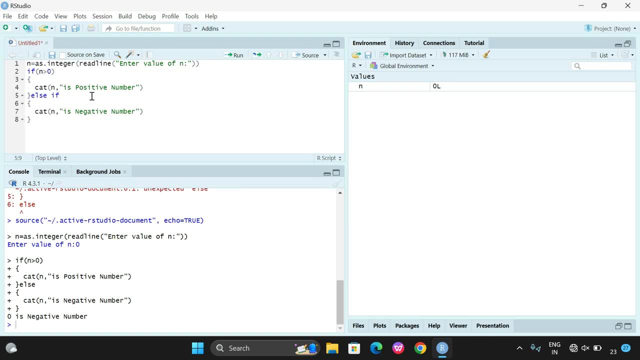 negative number. So here we need to check one more condition. So obviously we cannot write the condition at the else. So once again, just use a if statement and write down the condition n less than 0, and if both the conditions are false, simply you can give a else block. 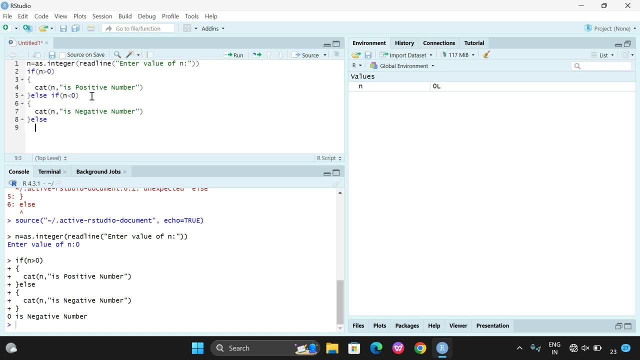 So else is also should be written at the end of the braces. So again you can write: cat n sorry, n is 0. So you can execute here. execute n value. If I give 0, you will get a 0. Right, so given. 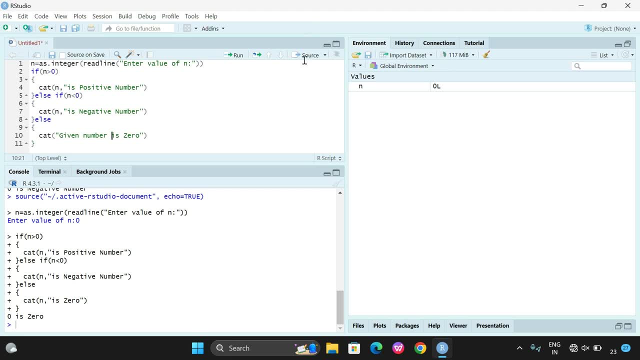 0.. Number is 0.. Right now you can observe, So execute: If I give the input as 0, we will get. a given number is 0. And if you give any other output, for example positive value, 10, we will get. 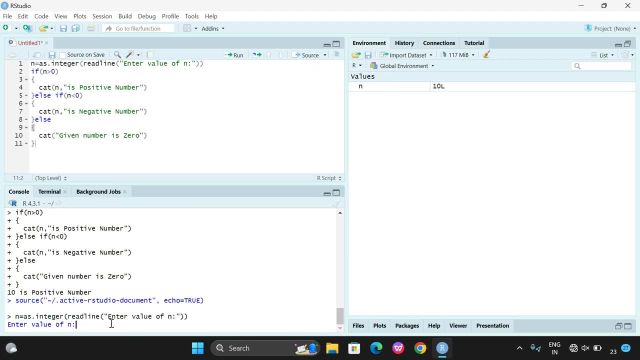 the result as a positive number. And if you give minus 20 and the result will be minus 20 is negative number. So here one thing we have to remember. So in the else block we should not give any condition. and if you want to check one more condition in the else we have to. 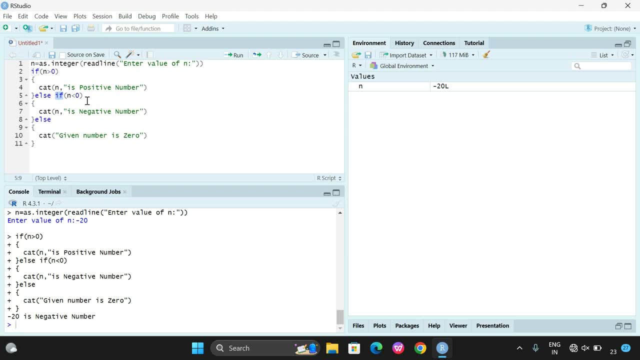 include if, and we have to write out. So in this way we can give a multiple conditions, We can check multiple conditions in a single program. So even though we are giving multiple conditions, only one block will be giving. one block will be getting executed. So here we have written. 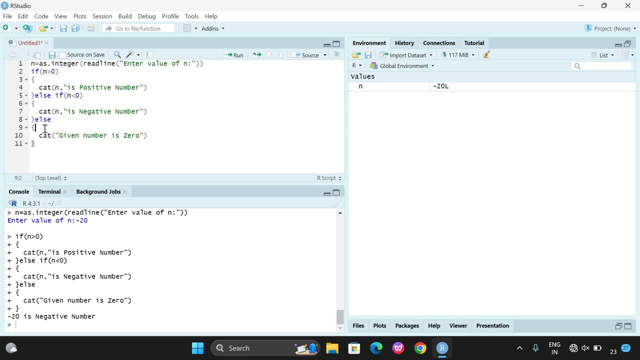 three blocks: 1, 2 and 3.. So even though we are writing three blocks, only one block will be get executed. So if I am giving the input as minus 20, see minus 20- automatically this second block will be get executed. Second block will be get executed. Right, So you can give a number of blocks You can. 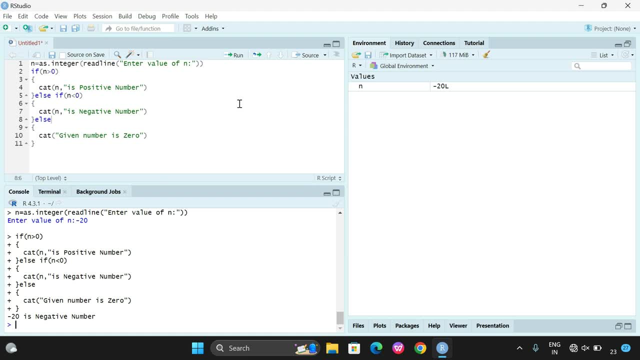 also write a number of conditions. Okay, Hundred conditions we can write, but at a time only one condition or one block will only be get executed Right. All the remaining blocks will be ignored. So this is then. this is an example, simple example, for else if ladder, Else if ladder. 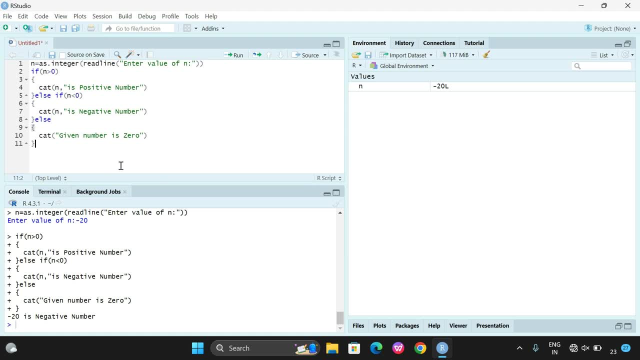 Right. Then next one is a nested if. That means inside the if we can also use one more if statement. So for that we will take the example of a largest among three numbers. So first of all let us take three values, So let us take A largest amount. three numbers is an example. 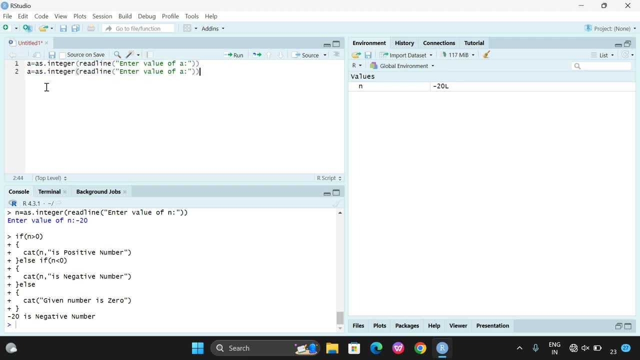 for nested if we'll take it as a nested. if so, I'm taking three values: a, B and C. so the first three lines give takes the input from the keyboard during the runtime. so we are having some ABC values. so we need to check first if a greater than B. 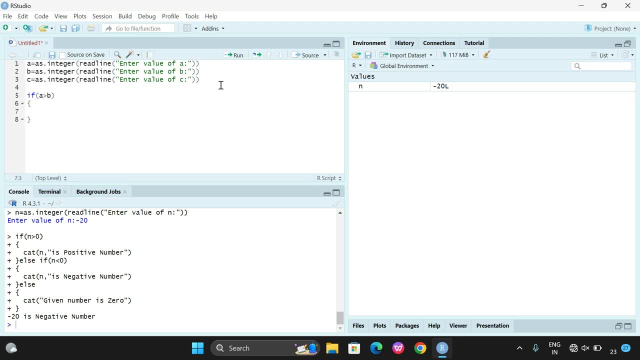 right. so whenever the condition becomes true, we can't say that a is largest or B is largest. okay, and yes, so this is the control enters into this yells. only if a is less than B. okay, only if a is less than so. here, if a is greater than B once. 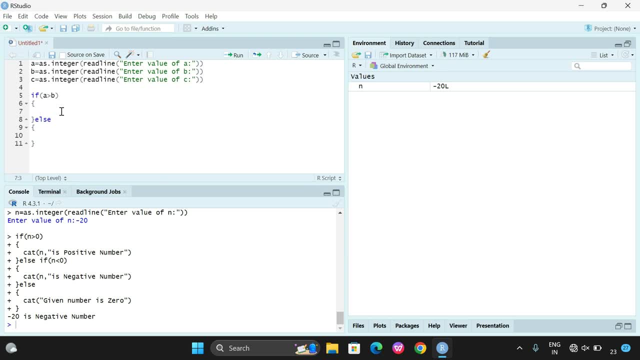 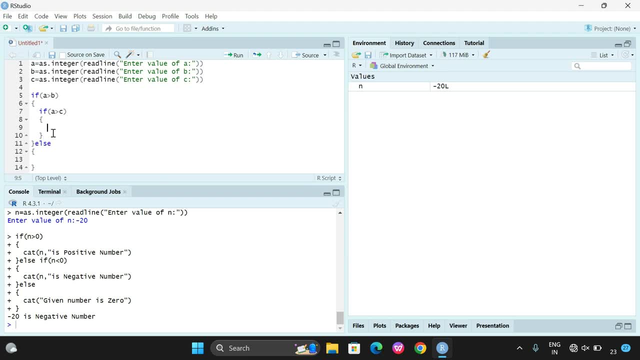 a greater than C. so again here will be having a tool. so far true and false. so if you a greater than B, okay, a greater than B. obviously a can be larger or C can be larger. if a is greater than C, is a will be largest in or a less than C. it. 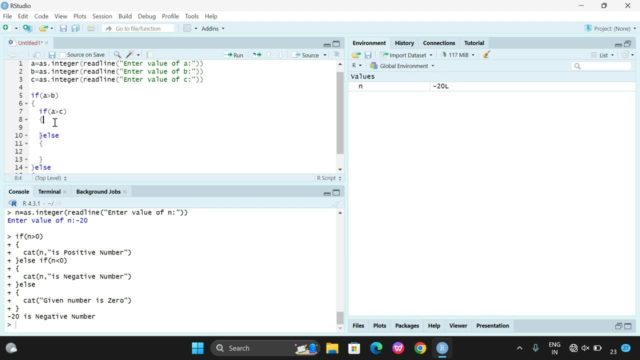 will be, C will be the largest element. okay, so here we can write it as so: whenever a greater than b, true, then this true block will be get executed. So in this true block again we are checking a greater than c. if a is also greater than c, we can say: a is larger, a is larger, and if a is not greater than c, we can say that so a is. 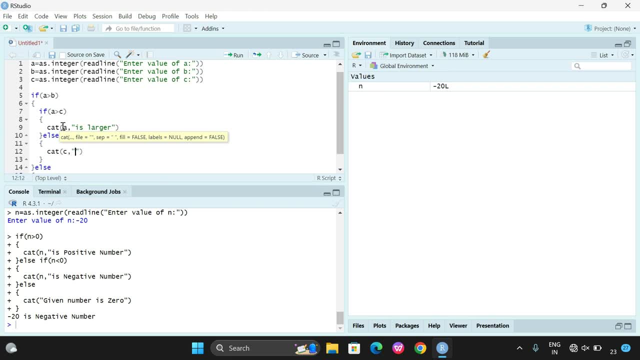 greater than b but not greater than c. so that means c will be the larger, c is larger. okay, and in the in the first condition, itself false. that means if a is greater than b is false, obviously it will be. a is less than b. that means b greater than a, right. So again we can check. 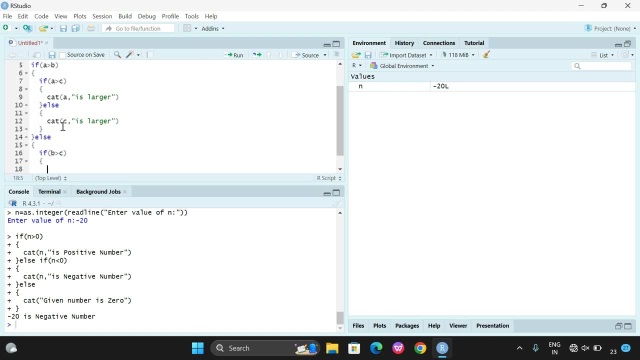 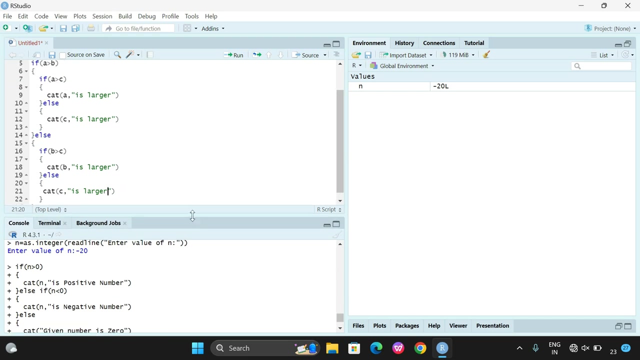 b greater than c. if b is greater than c, obviously we can say b is larger, okay, and else that means if, if b is greater than a but not greater than c, we can say that c is larger. So the simple code we can have as an example for nested if So, inside, if we are, 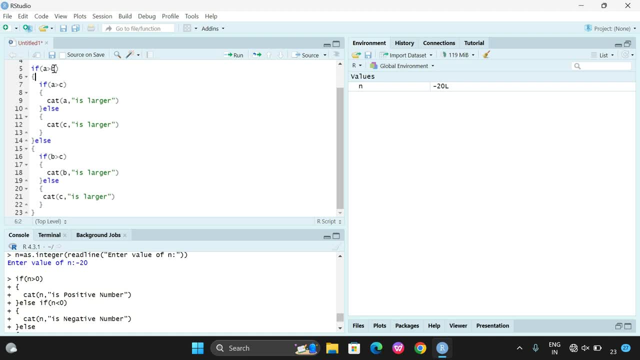 writing. so first we are checking whether a is greater than b and the possibility of this condition is true or not. So in this situation, if we are writing, so first we are checking whether or false. if it is true, then we can say that a is larger than b, and if it is false, we can say that. 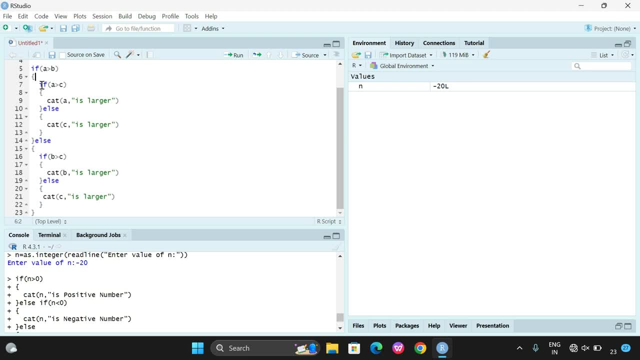 b is larger than a. so if the condition becomes true, so this will be get executed. if condition becomes false, this will be getting executed. so if a is greater than b, it is true. again, we have to check whether a is greater than c also. then only we can say that a is larger. so if it is, 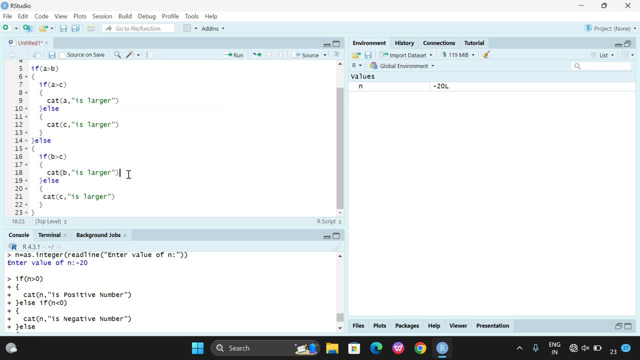 false, again, c will be larger. similarly here also. now we can execute with all the three cases and we can check. let us take some 10, 20, 30 and we can say 30 is larger, yes, correct. and again, let us take 10, 30, 20, sorry. 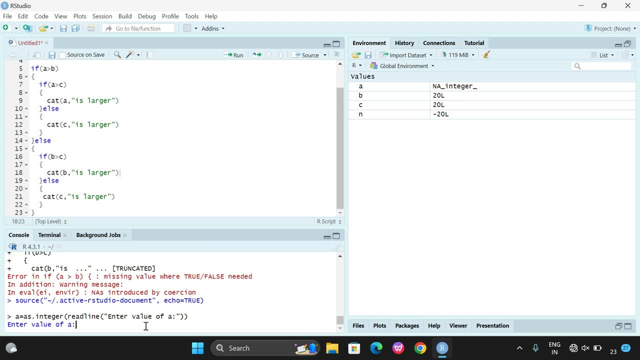 yeah, i'm giving the values: 10, 30, 20- again, 30 is larger. once again, let us take 30, 20, 10- again, 30 is larger, right? so we have taken the three cases. one in the first case we have given the third element.